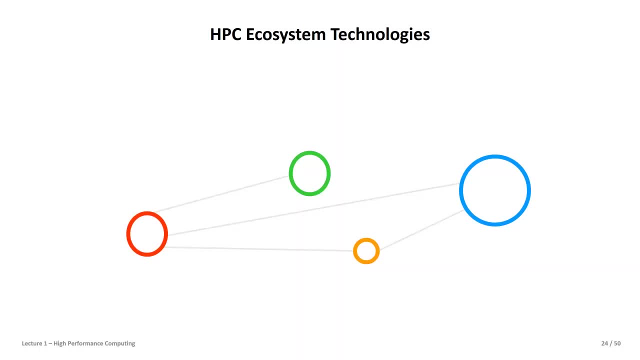 what are further terminologies? how you create such a system? You have something like racks and plates. You will see the evolution of HPC systems in this ecosystem. Some people will refer to this as a very, let's say, lively ecosystem, because we are always. 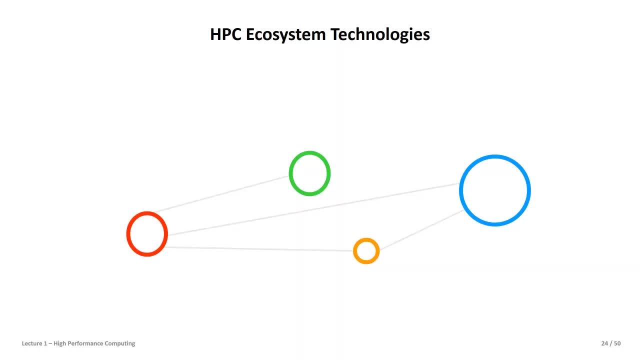 at the cutting edge of performance and there's always a kind of disruptive technology coming along, While in the past people have suddenly started to think that many core chips, like GPUs- we will come to In a moment- are really disruptive, They are normal kind of modus operandi today. right. 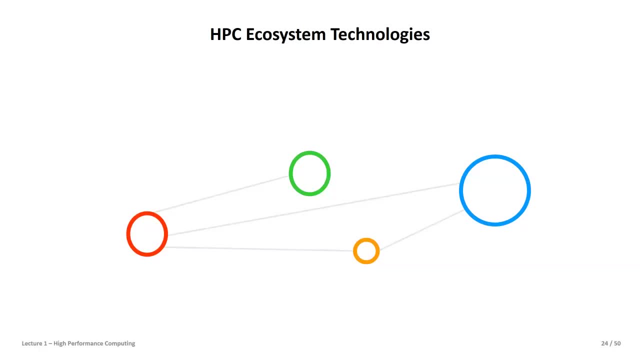 But today people will much more think now that quantum computing, neuromorphic computing that you maybe have seen in the video, basically also as one of the modules. these are now the things where we think that is disruptive technology which will shape HPC in the next five to 10 years. 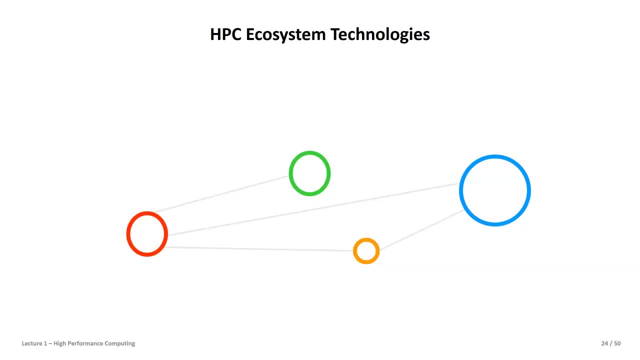 So that's quite an interesting art, so to speak, an art of bringing really different pieces together. You had seen the four building blocks, So let us look now a little bit into the HPC ecosystem and all the technologies. We have started really the course with kind of Unix. 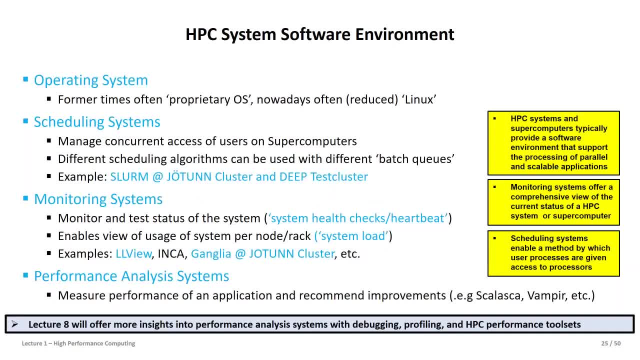 And with this you don't really have pure Unix. there You would have CentOS and maybe other reduced Linuxes. That's not the point, But usually you would have a Unix operating systems. We see Windows HPC clusters coming along, So also here and there Windows are basically HPC machines. 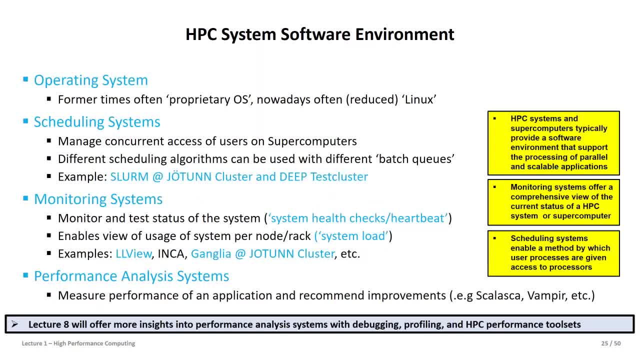 But they are, let's say, not really the majority. What you will see throughout the course is that such a HPC system is not yours alone. They cost usually lots of money, lots of millions, in the idea of jewels that you have seen in the video. 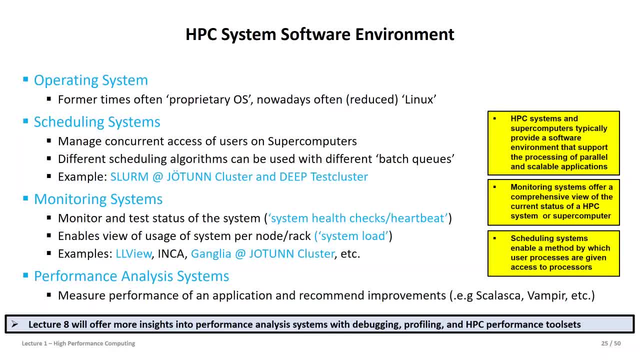 number one in Europe, But also U-turn and also even the deep test cluster has, let's say, lots of GPUs here. the deep test cluster This already costs. So you usually have that. these supercomputers and these HPC machines are kind of shared. 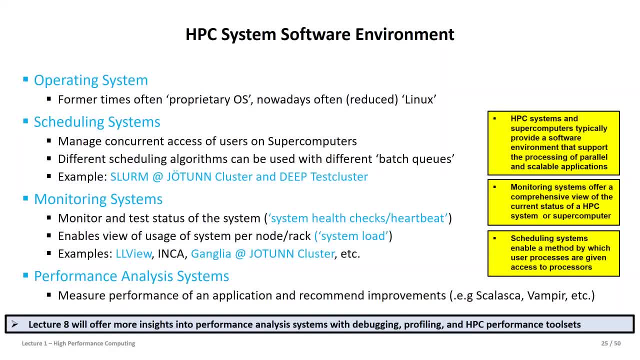 between different user communities And with this you have to have one system- We call them scheduling systems- that schedules different users, different algorithms at certain point of time in a queue And then the queue and the scheduler. that is basically this technology like Slurm. 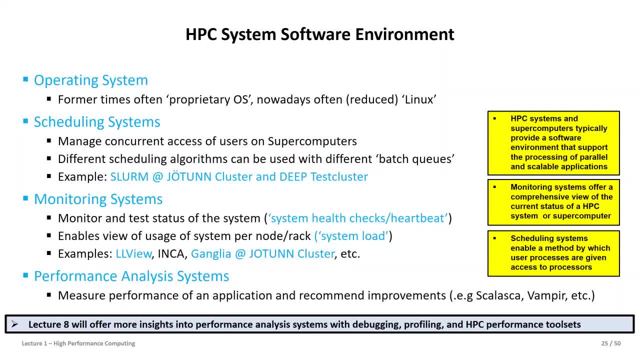 will then make sure that, firstly, it's get, let's say, to the right processors at the right time And, of course, that it's not overlapping or, let's say, interfere with other users and their jobs. And with this you can imagine this. 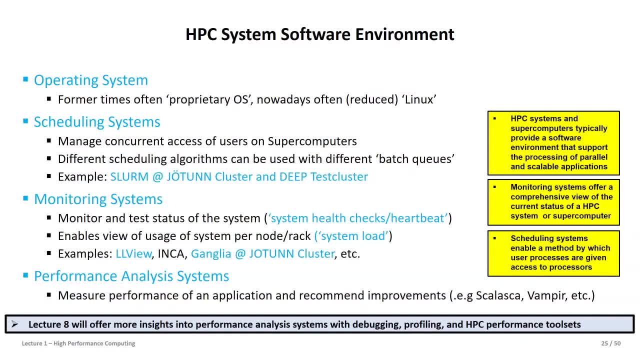 is a very important HPC system software that we will come again and again Also, particularly in my practical lecture 1.1 that I will provide you next time, where we look a little bit what that is, what a scheduling system is and what it doesn't mean really to have this batch queues. 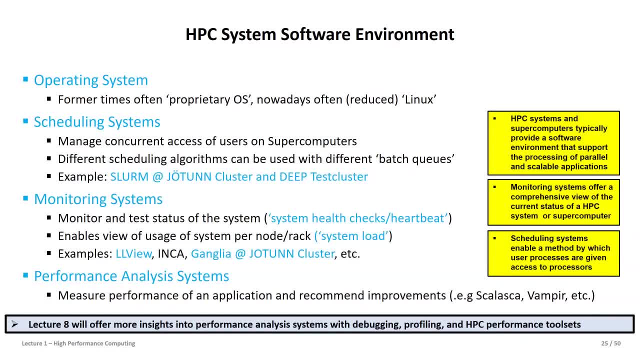 Now, when you think that this HPC systems are quite complex systems- you have seen networks, different racks, lots of CPUs. you need some monitoring system, not only to see how much, How much users are there on and what is the system load. 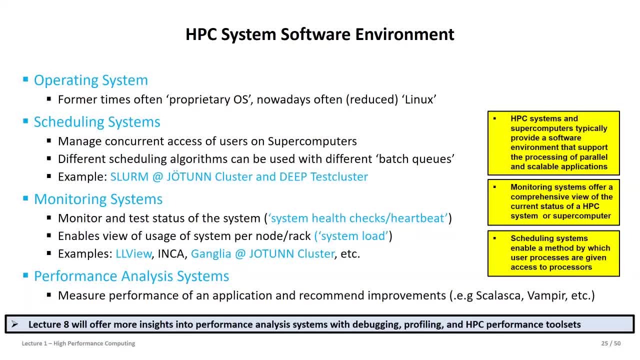 Also, what's the status of the system So? are several CPUs broken? Is a network interconnect not working? Is maybe the file system down? All of this are referring to some way of a monitoring system that is always required, And then there's a different part in the HPC system software. 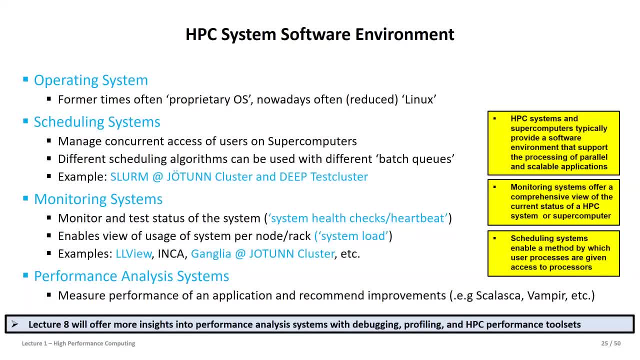 which is really then related to a big part of it, which means the performance. So you would have lots of programs that help you not only to understand the performance of your parallel application, but also to significantly improve it. There are tools like Skalaska and Vampire. 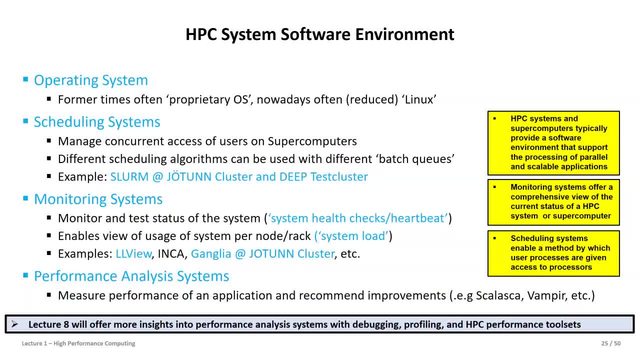 we will look into Lecture 8, when we think about the parallel performance analysis, which goes much more broader than just debugging and profiling, maybe your systems, You have really analysis of patterns of different performance problems, And we will come to this then in Lecture 8.. 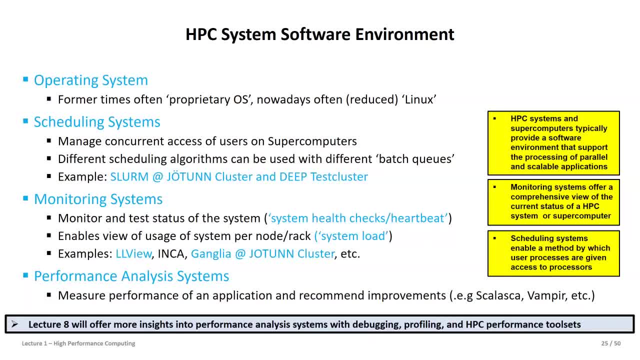 But all of these HPC system software parts you see here are kind of a key requirement. 1.1: You will rarely find the HPC system starting from U-turn. It had basically all of these two. what's really cutting edge of jewels, these kind of the really required. 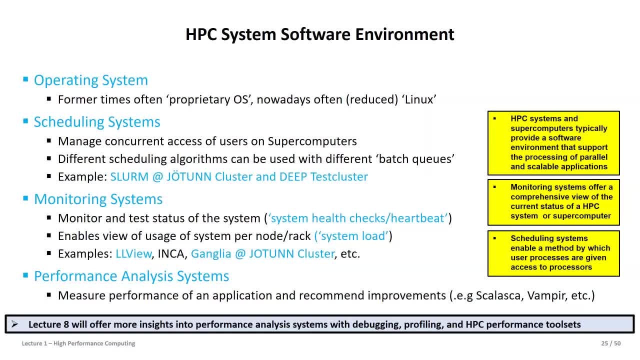 systems. While performance is, of course, something where you can argue, if you are trusting that your application is already perfect, you can always think about the placement then on your software, on these different systems might be having also performance issues. It's not only your application. 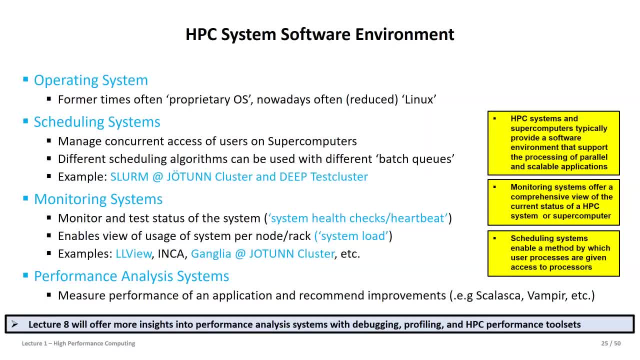 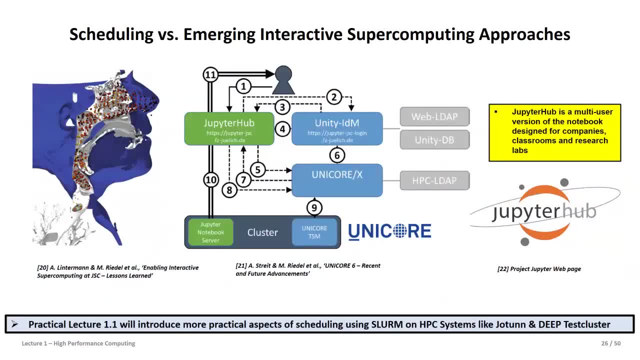 It's maybe how it is differently executed in parallel. So still worse. looking in performance analysis, Right, When you think now about the scheduling I said, you would think like maybe some of you from the data science domain, particularly how I compute this thing when I want. 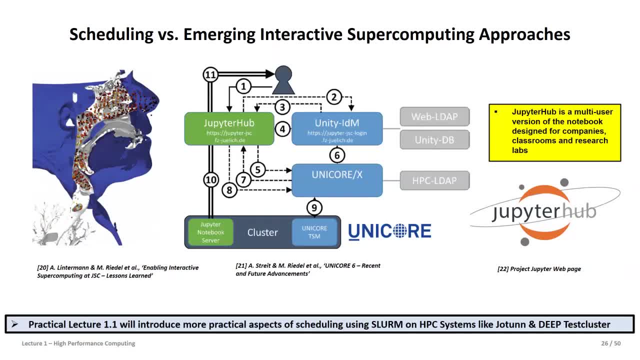 to have, let's say, my typical Jupyter environment. right, I have a Jupyter notebook. This is quite attractive. We not only do it in our complementary cloud computing course a lot, we also do it in the data science community as large. 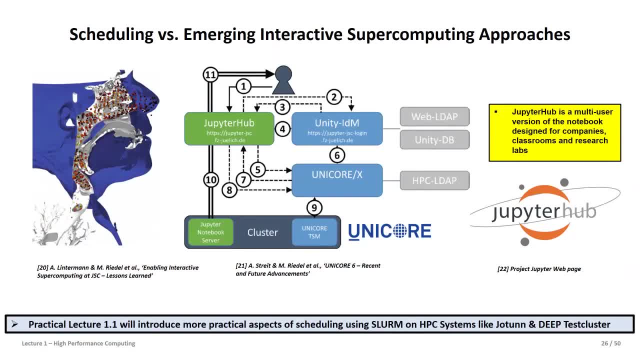 And there you want to have a lot of data science. You have a GPU directly at your disposal. You want to have directly, let's say, an execution. You don't want to wait quite long of time. However, in these data science approaches, 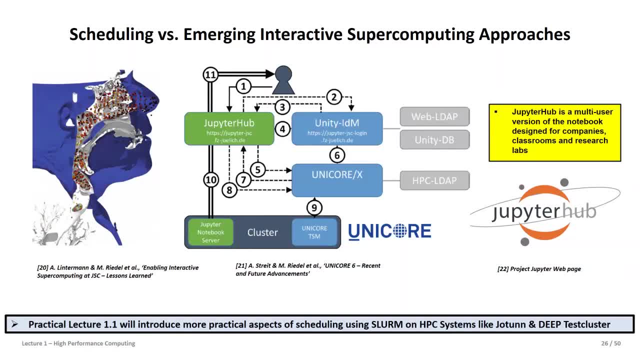 usually you would have- especially if you're experimenting with some data science tools- often an idea to not directly, let's say, have 96 GPUs together to really scale largely. You maybe have smaller jobs that you don't really require to have in a batch mode, so to speak. 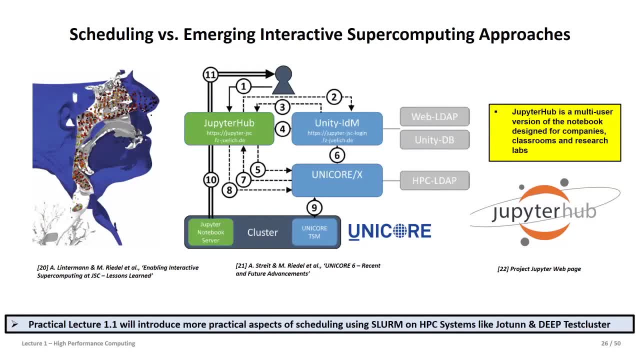 Here We talk about this interactive supercomputing which is actually becoming more attractive more and more, And here's one way how you can access such a system. You don't need to know exactly all of these different steps, But in order to, of course, basically have a Jupyter hub. 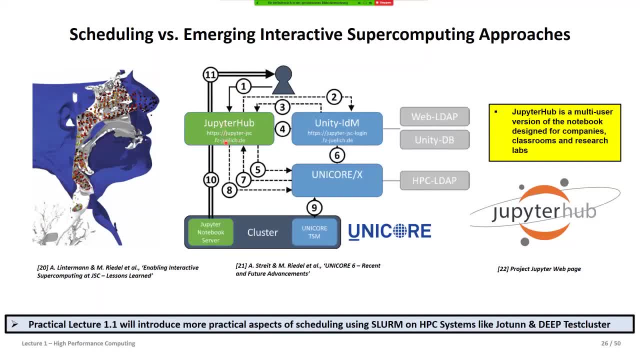 or a browser-based access really to a computer like a supercomputer. you need, of course, also identity management. It refers a little bit what we learned already of SSH, of username password And one technology that you have here. 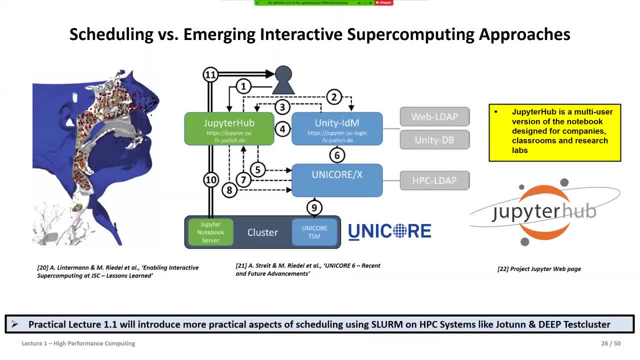 that is actually realizing this is Unicore. It gives an access, together with Jupyter hub and basically then the Unity identity management for this And we will have some examples in the course when we come basically to data science problems using HPC. But it is a larger area of supercomputing really. 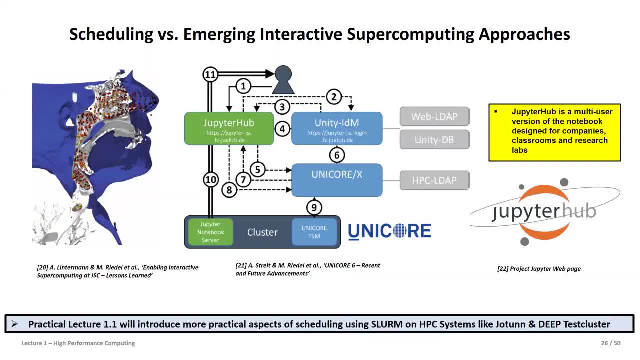 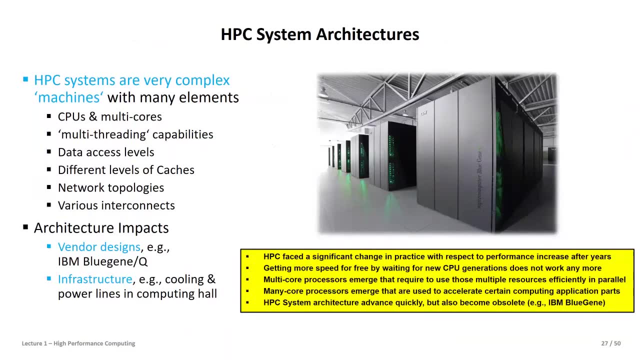 to make it more interactive these days to maybe steer then parts of the supercomputing simulation. So it's a little bit of a challenge to be able to do that during the run time and to have an interactive channel Now when you think about HPC system architectures. 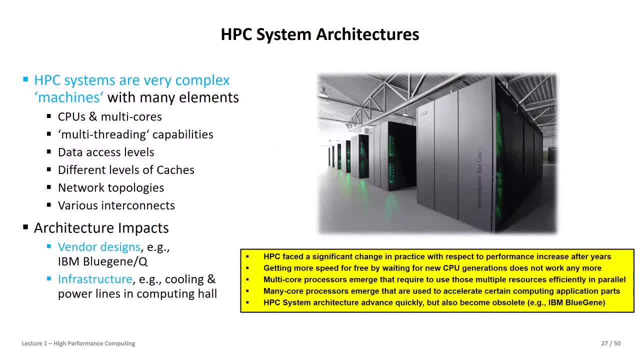 let's come back a little bit to this with a broader picture. We started this in multi-course, But what you see today is kind of two things. Firstly, very old architectures quickly running obsolete. They're going out of date. They have been quite around for some time. 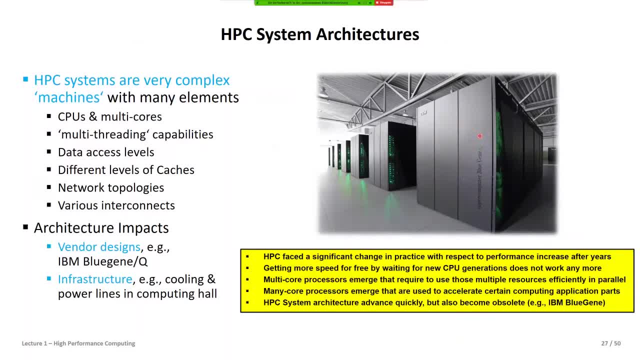 And you see here This is a supercomputer, Blue Gene Q, which was a very strong systems in the past, based on long history of a Blue Gene L, of a Blue Gene P and then a Blue Gene Q. So you see, basically, 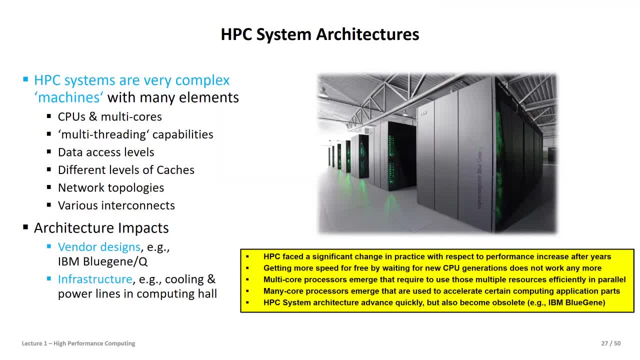 a complete line of a vendor of supercomputers, And they had also different specialities to program them. When you go to different systems, this will be the same thing. However, the basics remain the same. You would still use OpenMP. 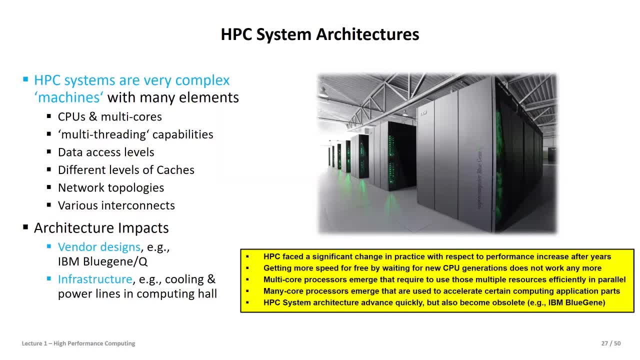 You use basically MPI, But the tuning capabilities of multi-threading, for instance, or basically, of course, in newer versions of this, the ideas of interconnects, network topology supported and, of course, the advent of many core chips. now. 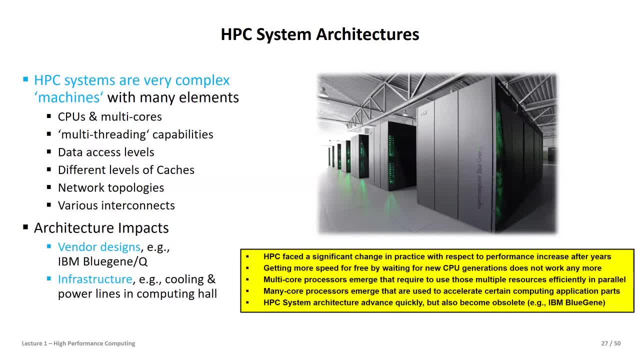 they change the system architecture significantly And with this we have really an interesting, let's say, momentum in these HPC system architectures, so that it has quite some impact that this technology is changing all the time. And we will see when we look a little bit more. 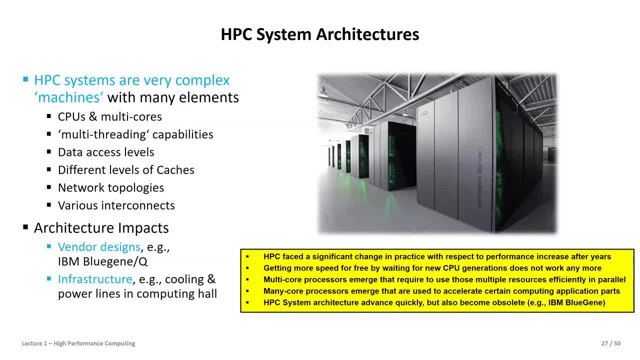 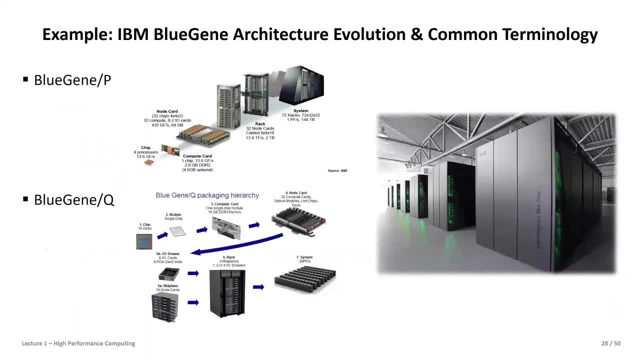 about many cores also, how quickly they change over time and how quickly they change over time And of course, the idea is of changing always technology and how it impacts actually a quite established field of HPC quite significantly. I brought you this example saying that, of course, 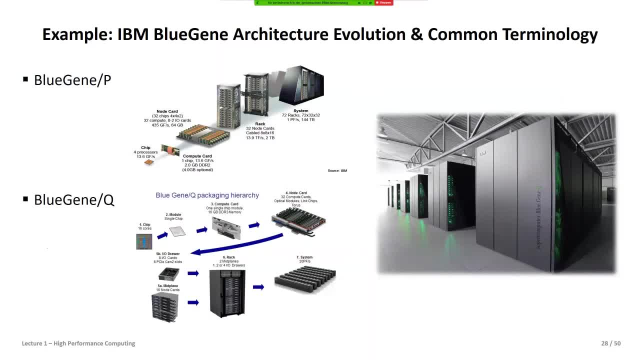 we said that the supercomputer Blue Gene Q is kind of obsolete. There is no Blue Gene series anymore from EBM, So but the message I want to leave you on the table is that, of course, some of the terminologies still remain the same. 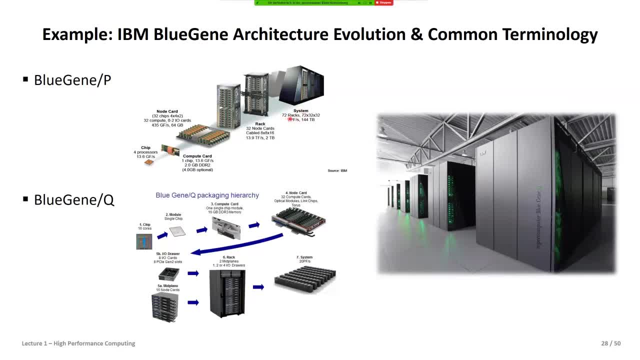 And most of it is, of course, in the same form, which is usually compiled as forms of several racks, And a rack is sometimes hidden. You barely see it, But essentially these parts here of this is all in different racks And meaning a rack, then, basically. 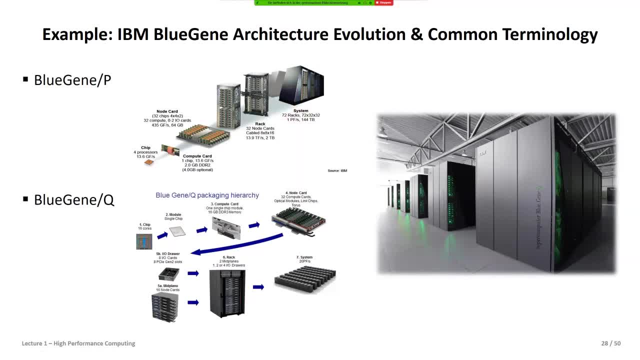 is a very interesting, dense way of putting lots, of, lots of, lots of cores, And they are usually in so-called note cards organized, which are really, of course, all of them have a very good interconnect together. Here is also where it starts to think about cooling, but it's something what we have also in later parts of this lectures again revealed. 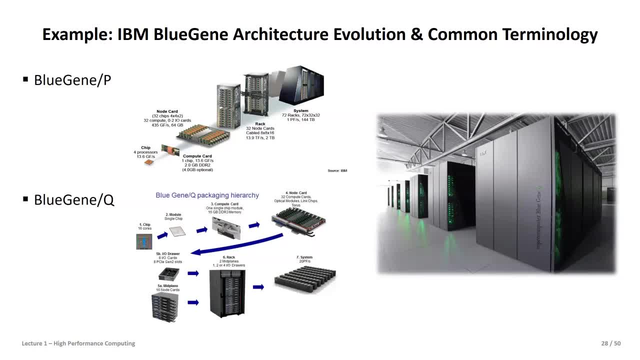 In former times lots of air cooling, thinking about heat coming out and coal- basically cooling- coming in. Today we have more liquid cooling and also even that the, let's say, the heat that comes out of a supercomputer can actually also actually heat up buildings today. 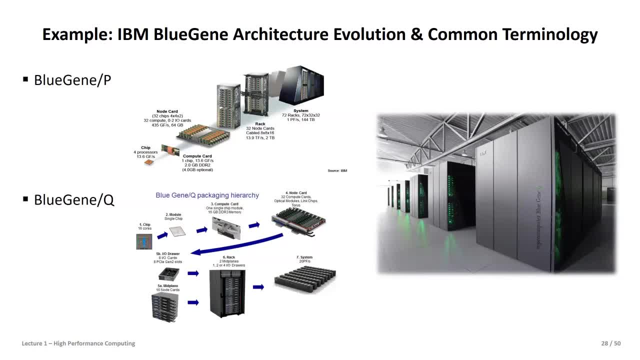 But this is not really the key idea of the lecture today. Here is rather to think about that. you know these large systems. still, the key ingredient on the lowest level is a processor, And this is important. There's no difference than you would have in your laptop, in a sense. 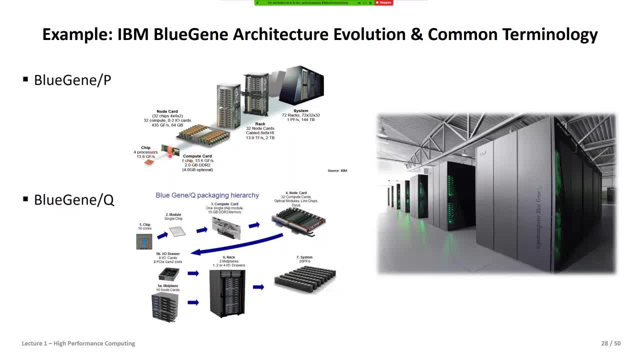 Of course these are specialized chips that go to specialized compute cards that then very densely get together on so-called note cards that you then can include in the rack. And you can imagine So many compute chips with you know that really create lots of heat, so densely, basically put in such a rack. 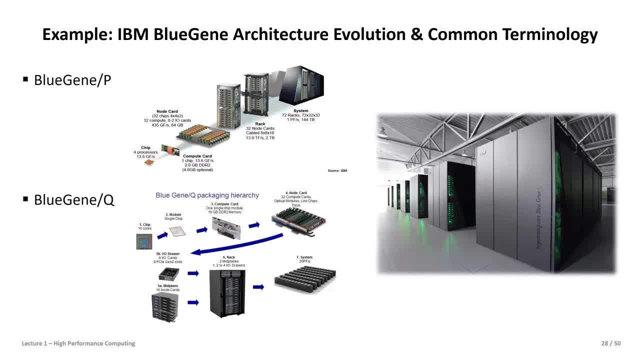 We will see, when we have the opportunity, hopefully, to go in one of our, you know, computing centers, that there are lots of heat coming out And basically this is a key consideration, of course, how you do the cooling and because the cooling also can have lots of energy impact. 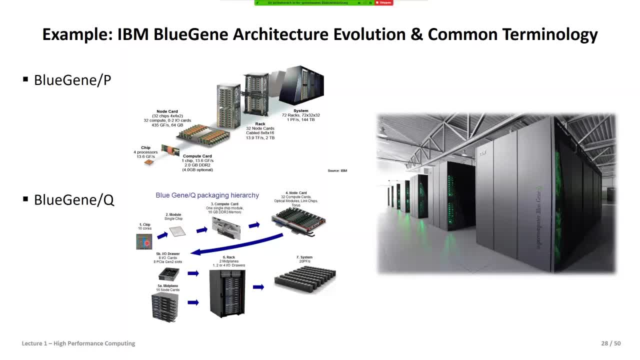 Right, And with this you see that even the smallest chip can Then actually be the Lego building block, if you want, of a very, very large system with lots, of, lots of racks. And this is the idea that we have seen, for instance, and also when these pictures were evolving to more and more racks that actually filled them more and more of a whole. 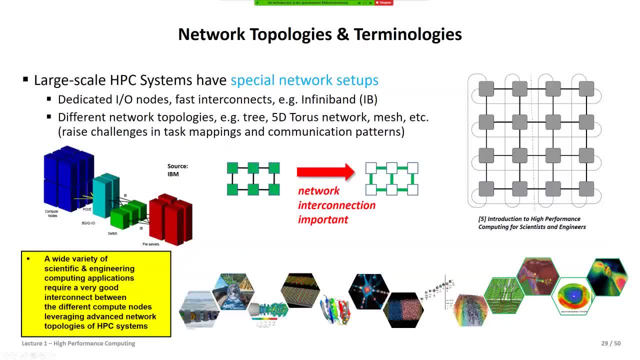 So, but the computing is just one part of it. We also said HPC is defined by really having extraordinary network topologies and interconnects And this by far today means InfiniBand. We have basically Mellanox often in these systems that have a very good network. 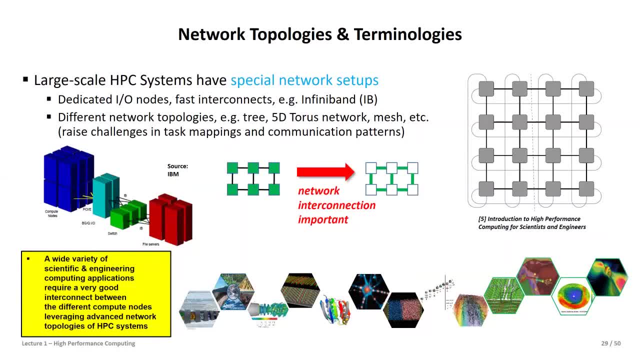 We have different topologies So we cannot only communicate basically to, let's say, my left and right neighbor. There are also different dimensions of topologies And we will see when we go through all of these different applications here today in later parts of the lecture. admittedly, when we look a little bit more to the domain- specific sciences that leverage HPC- 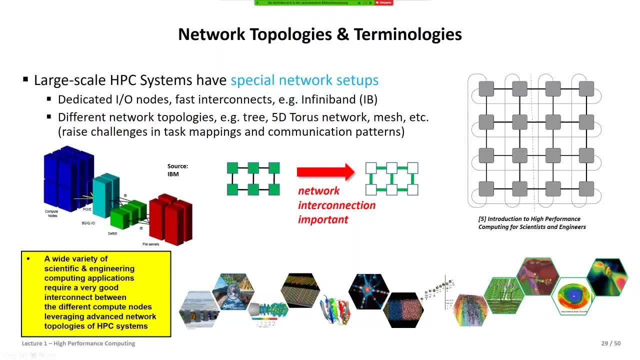 Right, Right HPC systems, that these network interconnects are really exploited. You have already seen in the video the Vulcan ashes. They have seen how jewels is used from the scientific applications. All of them, for instance, make nearest neighbor communication on, basically then have another way of communicating in parallel to maybe a couple of cores or basically different nodes that are basically far away. 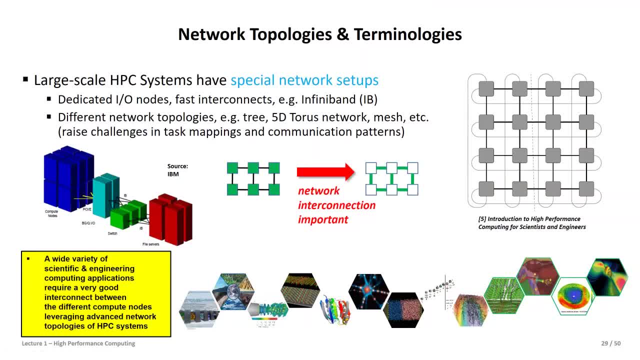 However, in order to do this, you really need Good communication patterns and you need, of course and really, the hardware really dedicated, fast interconnect, including, of course, and not forgetting that you have data. So here's an idea how that could look like. 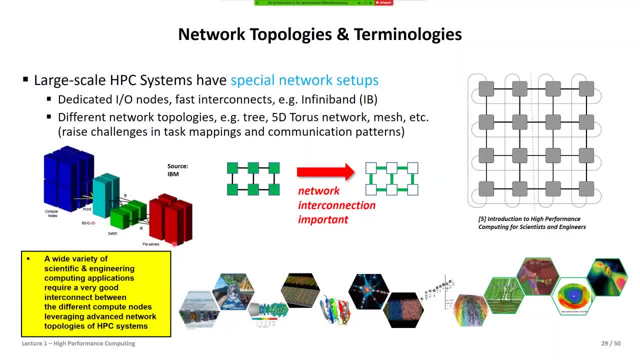 You have lots of compute notes, but you have to think about that. There's also file service and lots of data And by today I think this is more the challenge that you have still of having kind of a bottleneck from the computer, the file service we see. 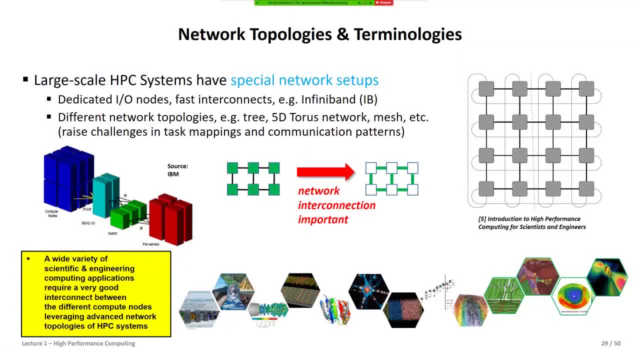 We have there a parallel file systems. We will also have in one of the lectures, much more revealed and also being slightly part of your assignments. But there's of course a big problem of when you have remembering, remember maybe the 500,000 cores which are in machine. 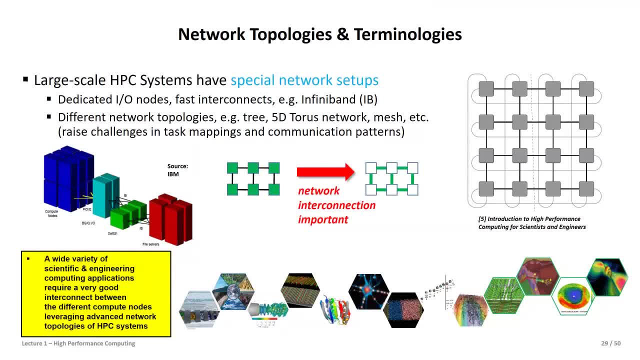 So how do all this compute cores right to disk? And there you need to be again certain, let's say throughput, which again falls back of course. now to the network interconnect, But also basically, what type of notes you have. 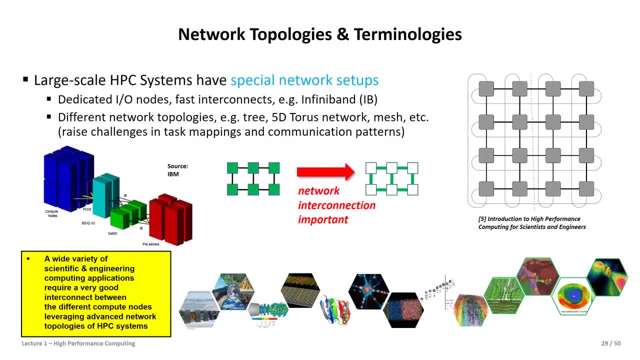 You can have dedicated notes, for instance, So this will also come in subsequent lectures, right, But the key message is really: HPC is really driven by this, by having also then the main motivator of HPC systems. We don't do that for Bitcoin minding. 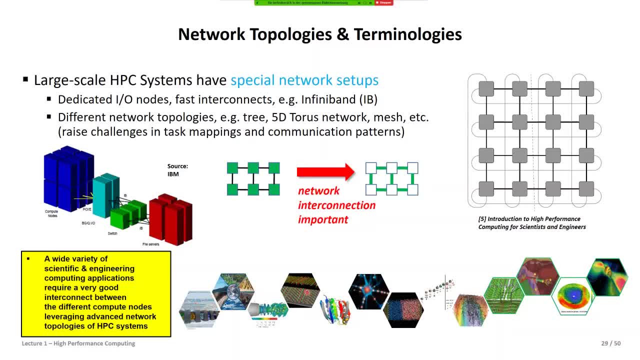 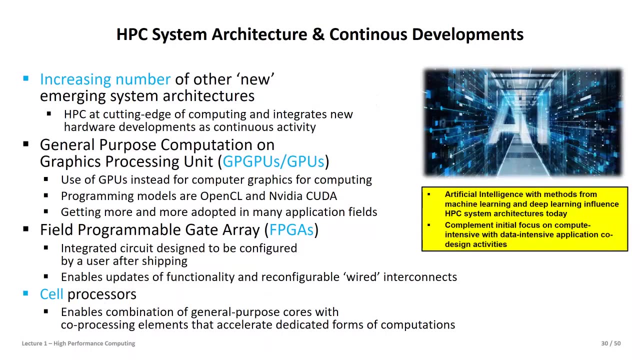 We don't do that for fun or for gaming. We do this for the scientific applications that really require such a communication pattern, such good network topologies. Now, when you think about the system architectures and continuous developments, I would like to refer to a massive, massive way of possibilities. 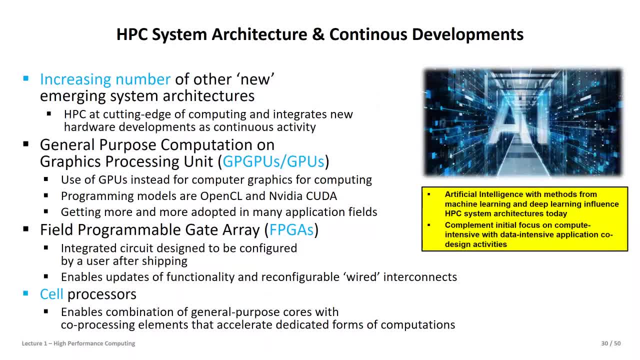 You have lots of ideas of cutting edge technologies can maybe be integrated. One interesting example is, for instance, network attached memory that we have just essentially in our research project, which is not on the market Right. We have one paper about it. 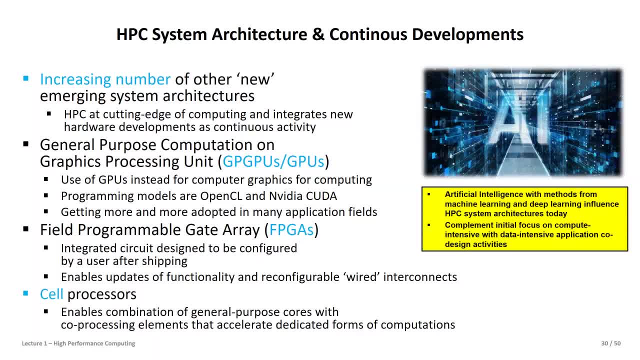 We have by experimenting with it. What does it mean to have? We have a memory on the network instead, closely to the ship. You maybe can share more data with other users and in a more high-performance manner than just putting everything to disk. And you have seen the non-volatile memory coming into the game these days. 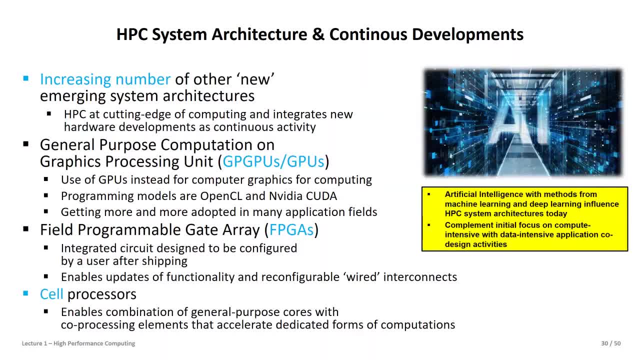 We have seen the many core chips coming very, very quickly into the game of rising from, let's say, computer gaming into scientific and engineering computing with an extraordinary pace, with one vendor that you all know, NVIDIA, being, let's say, a major market vendor today in this area. 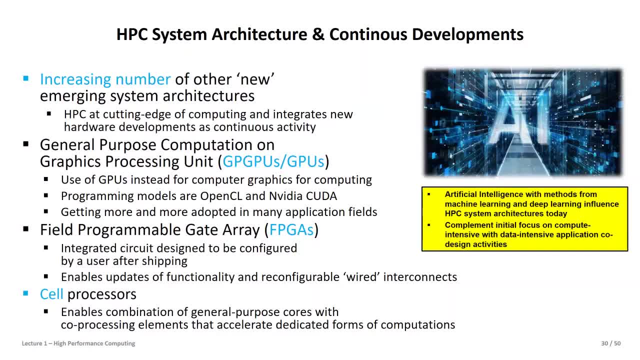 But, of course, influencing lots of system architectures. You have seen Jubilus is also using NVIDIA technology, as also using lots of the US systems in the top 500.. There are more, let's say, specialized systems, What you could do with the so-called FPGAs. 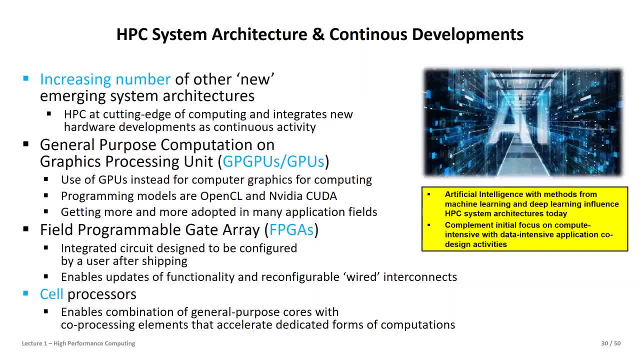 And this would be almost kind of programming them and, you know, kind of understanding them. really another lecture series really, But think of them as really interesting connections and like a CPU. but they can be much more reconfigured and rewired, essentially in this integrated circuit. 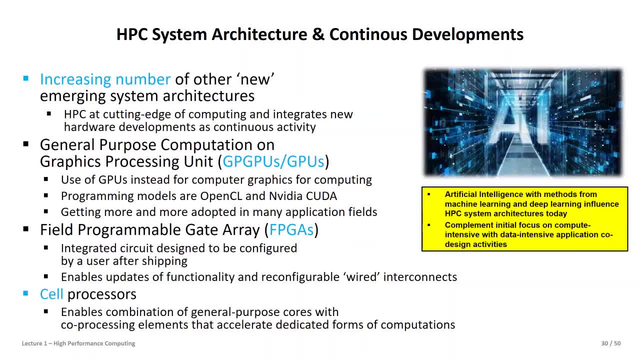 It's more technical, so it's not really part of this course, but of course, something you could think about. And then we have seen in the past also certain cell processors which had quite interesting capabilities. But the key message really- and that's why I brought AI today- is really that the system architectures were basically driven. 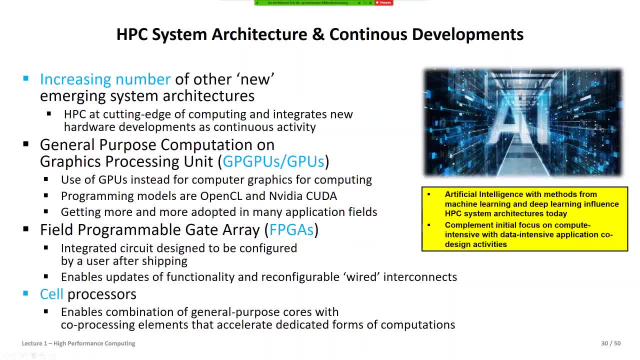 In the past much more by, let's say, physical laws, numerical methods and different parallel applications or simulations over time of different parallel, you know, and physical processes. But today we really see an influence of AI. So AI is more and more using HPC, is contributing to the workload of HPC systems. 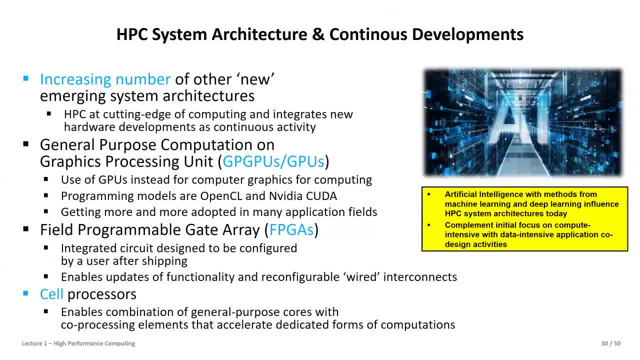 And with this you have a complete different requirement here and there, right, Of course, it's still compute intensive in a way, But it comes also To the point of being data intensive as well, while HPC applications in the past in the simulation of physics, also are quite data intensive. 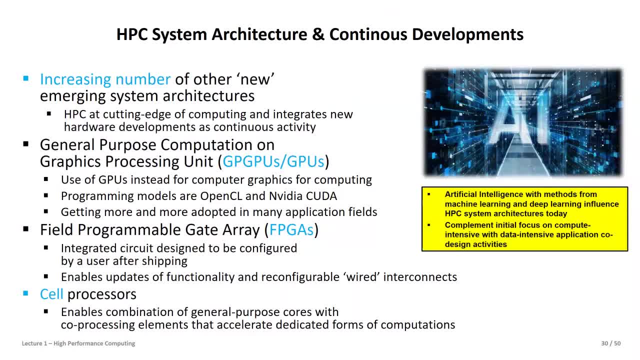 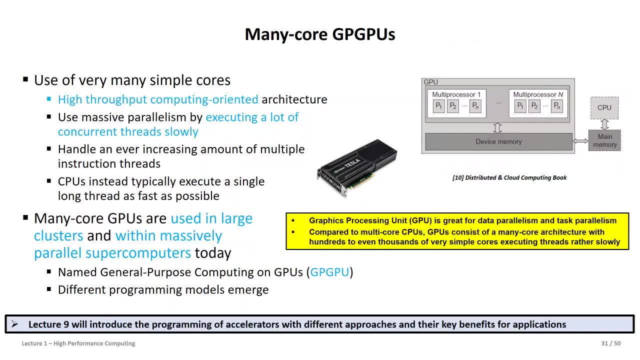 Here, the idea of using the system is, of course, a little bit different than we have in this physical situations. You analyze data- big data these days- and you want to do this in a very powerful fashion, And this AI really has, then, given rise to many interesting aspects of HPC architectures. 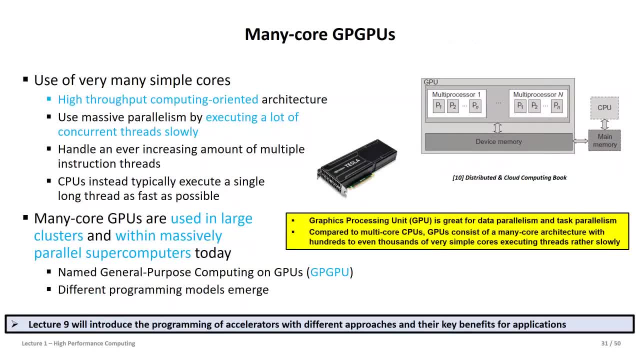 And the. So we see today, really, that the shift of computing is more and more happening from CPUs to GPUs, And this is now a completely different idea how you have such a GPU. Let's look a little bit into this GPU device to really understand it. 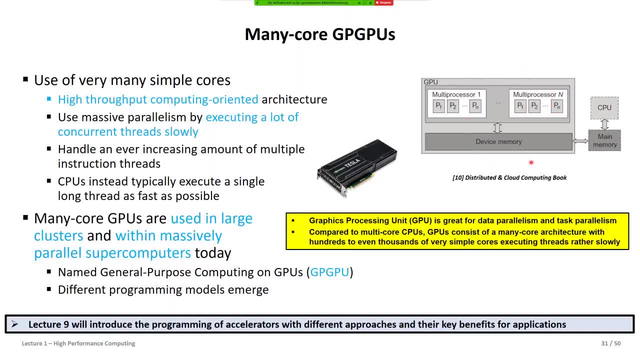 First of all, a GPU- is important to notice- cannot really operate on its own, So you still need a CPU, a general purpose CPU that we have seen in the first part of the lecture, which could be a multi-core chip, And the way how you get data from the CPU to the GPU is usually through the main memory and then through the device memory, which is considered to be today still kind of a major bottleneck or a challenge really to work on. 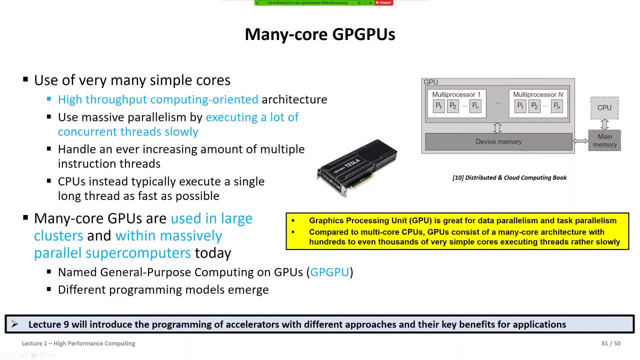 There are different solutions for this, but of course this is kind of the major limit. if you want to have, let's say, many, many GPUs interconnected, You have to have not only the memory very well connected but also think about the bypass of, let's say, going through the main memory. 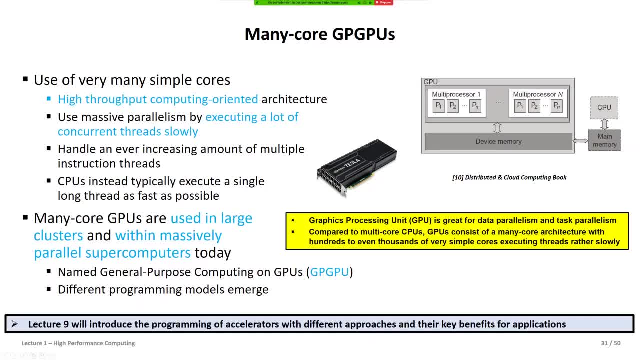 We will see in the GPU lecture. there are certain solutions to this with NVLink and we switch from NVIDIA or the GPU direct interface where you can kind of directly go to this memory space. But this is something for this lecture. then in lecture nine, 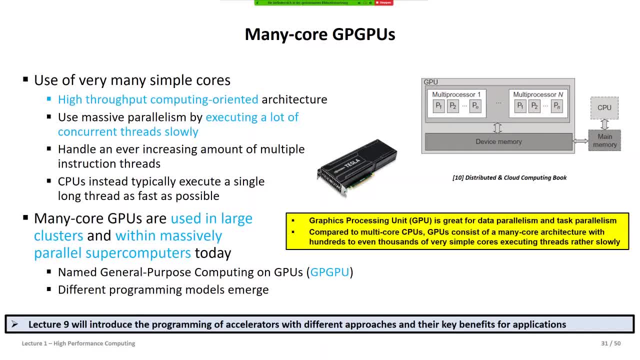 Here to understand it in the beginning of the course. it's perhaps much better to understand that actually, in comparison to have the multi-core CPU, a many-core chip like this GPU has really many, many, many processors. And now you would argue why they don't. 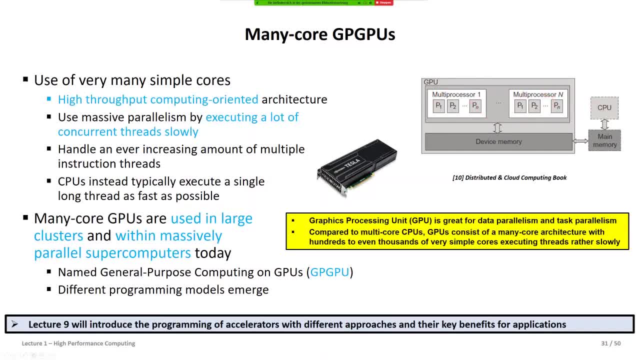 You would argue why they don't do this with a multi-core chip and just having also there more and more processors. And again it's about the frequency, the clock frequency, the heartbeat of the CPU. Here we talk about many moderate processors with a, let's say, not so high single-thread performance as we have in CPUs, but hundreds of them. 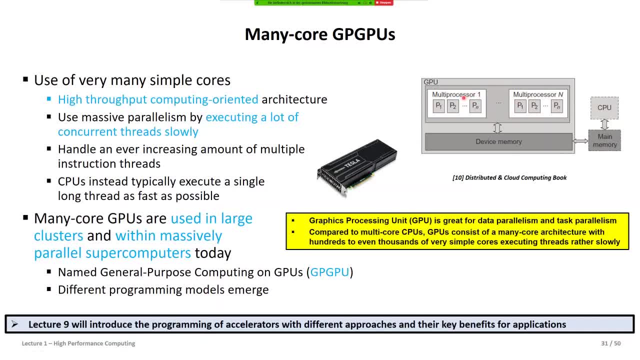 So here the emphasis is on throughput, Do very much calculations in the same way, but with many, many hundreds of threads. So in a way, A little bit, you could say it's shared memory. right, They want to have, you know, always have the device memory and then do the same on all of these GPUs. 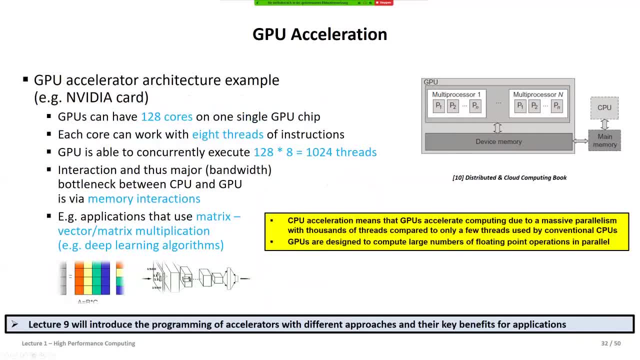 So let's see how that is, as an example, to be seen. You see here already the number of an example with a, let's say, older NVIDIA smaller card, but still very relevant, where you have already 128 cores on one single GPU chip. 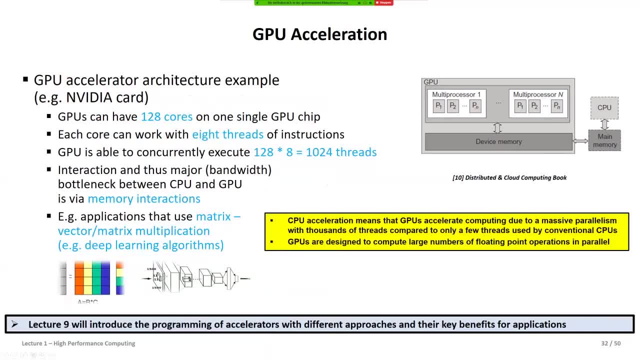 These days we have much more of them. But the point is to understand That these threats can all be working in parallel when you have, let's say, different here- a number of threats working on these different processors, leading suddenly very quickly to a large amount of threats. 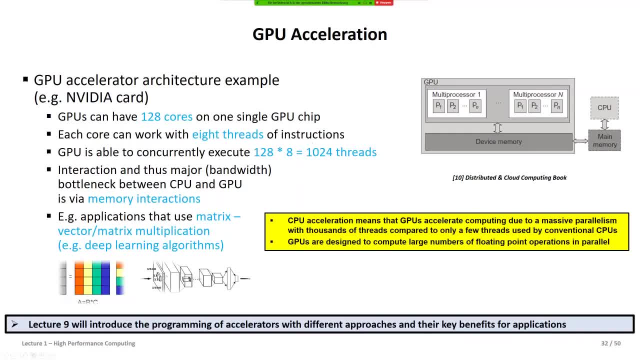 Of course. admittedly, we say they're not very powerful in terms of computing right Compared to a CPU. Still, we have a lot of threats can that can work on parallel And this has several different advantages and you can come to different workloads where that matter. 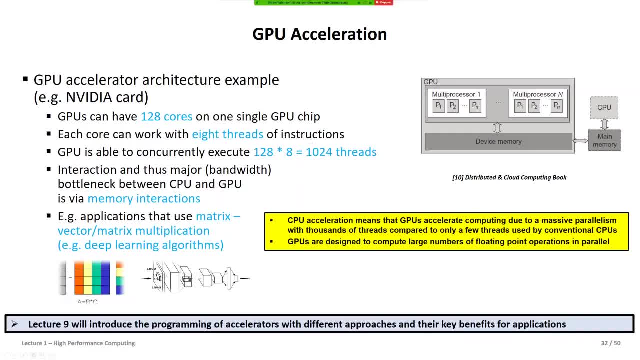 I think a very good one to understand This really here, the color coding, when you think about, for instance, a deep learning cutting edge network. we will have one lecture where we talk about much more about deep learning and also accelerators in this context. but think about there's lots of matrix multiplication, matrix vector multiplication happening in these deep learning networks and the way to understand GPUs would be here, that you would have this color coding of this mathematical principle, how you would do now this matrix and vector multiplication. 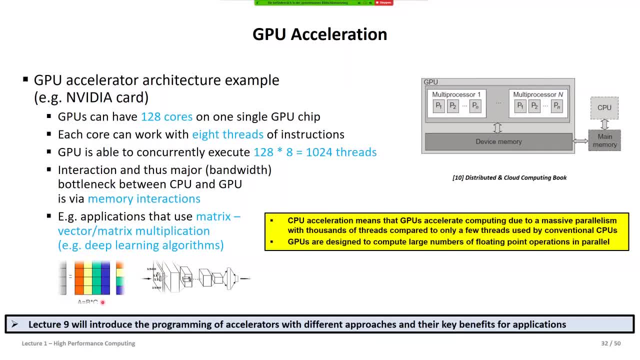 You see Immediately, When you remember a little bit from math, how that would look like to get the result to be computed. you can do this independent right from the other colors, and this gives you an enormous advantage. This means these can be completely in parallel computed without ever required to know essentially what the result of the others are. 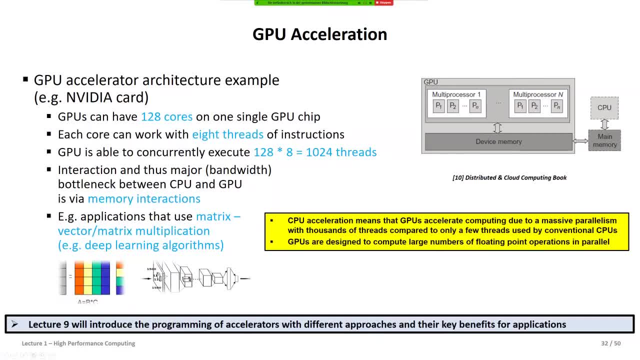 You just have a different part in the device memory, You put it there and you're done. But of course this could be all differently by threats, So you might have different methods, You might have multiple ways. you know you can go ahead and do whatever you feel like that, and then you can go ahead and update these methods. 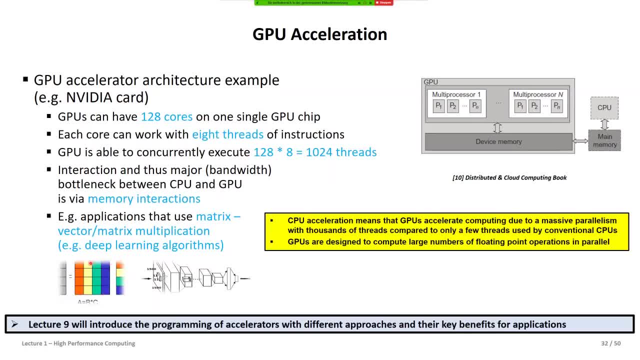 You can take one of these different tools and then, as I said, you could incorporate, like the metrics that you actually need to exit the GPU. Now, of course, I mean you think about cutting edge deep learning algorithms. These matrices are not in the order of four by four. 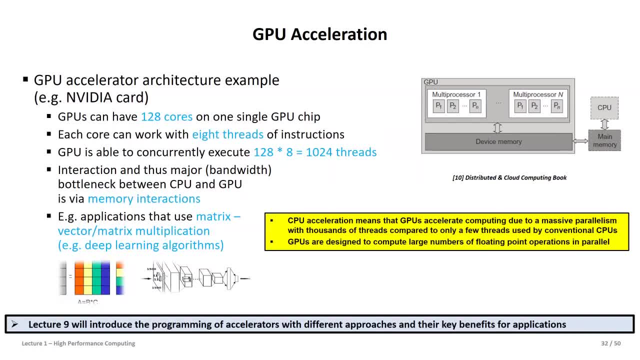 Here's the metrics. These are, let's say, multi-dimensional, They are much larger and with this, this power of really breaking it into independent parts- which independent is a very important part here- But doing the same calculation, Right, But we don't change. 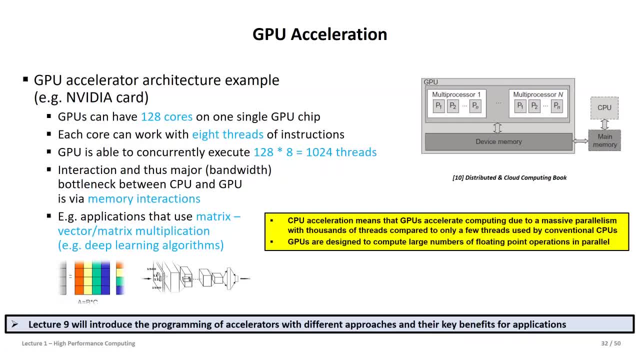 The mathematic principles, All the same adjust different data. This makes it so powerful, this concept of combining GPUs with CPUs. So we see here something which perhaps will never be the only way of computing, but it's an important part of computing and always will complement the general purpose of computing that we have more or less in the CPU to a significant part, as we see. 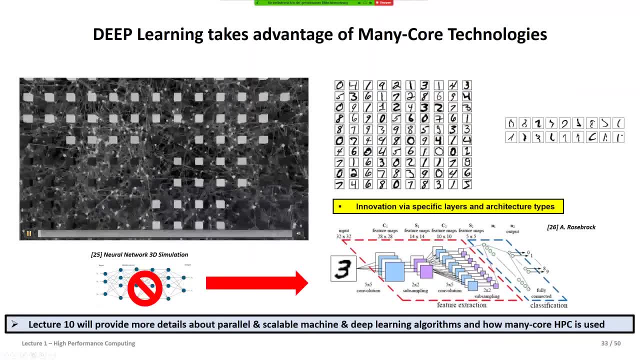 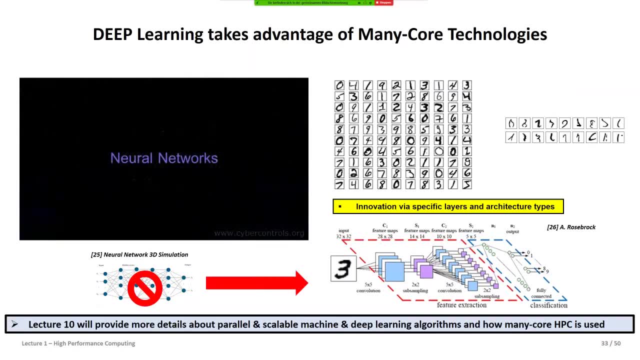 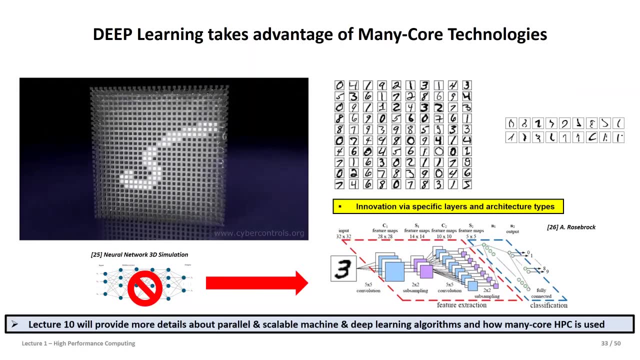 Just a bit more on deep learning, because it has quite an impact in that factor and I think many of you are not puzzled. what the heck does he mean by this? I'll give you a very quick example here, where you have neural networks which are basically learning then how you can basically recognize these handwritten characters. 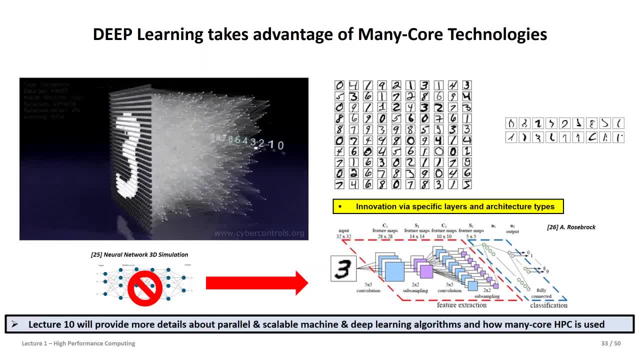 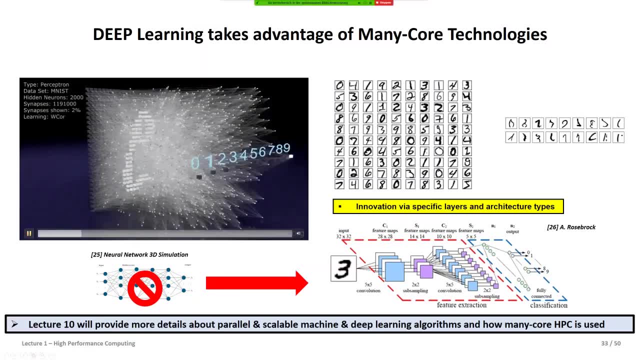 It's a very simple example, admittedly, but you see, a neural net has these interesting neurons all connected. Here's a simple perceptron and you can learn the weights, so-called connections, and they emphasize basically over time, iteratively, by going through. 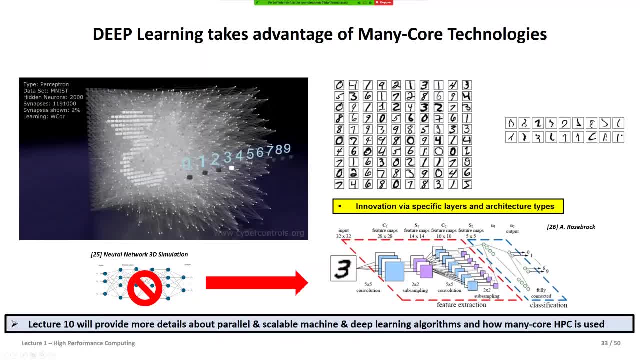 HPC systems so that you really are able, after the training, to recognize these numbers. Admittedly, this is a high-level statement. We will look and see how that materialized when we look at Lecture 10.. However, the key message is that, in order to train this, these weights of these connections, and when you go on to more larger networks, you see that the networks, the connections between all of these neurons become more and more important. 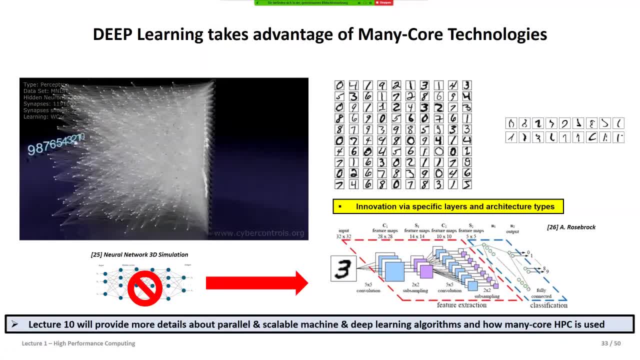 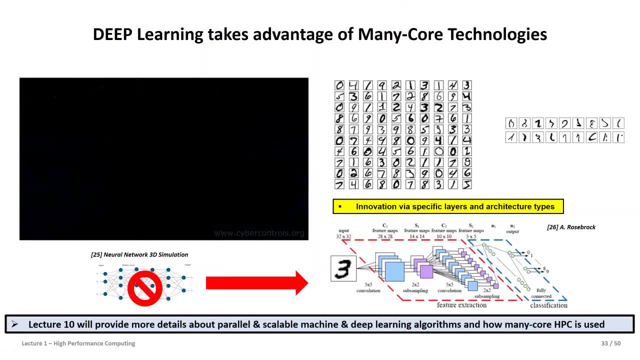 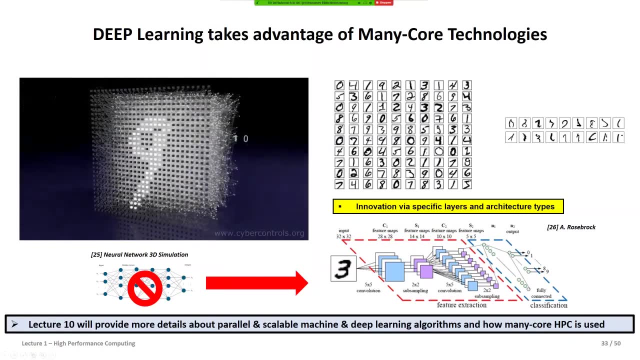 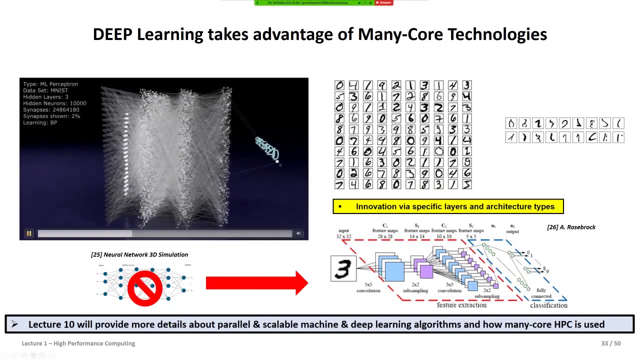 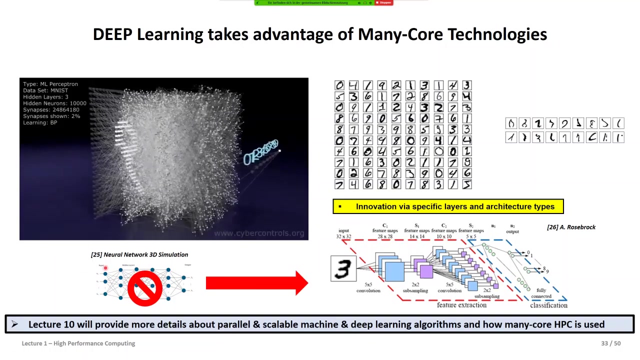 The Here you can now clearly see the different layers. I brought you also here a visual representation on the bottom where you see essentially these are different layers. we call them also artificial neural network. a multi-layer perceptron was having specific properties like a feed forward. 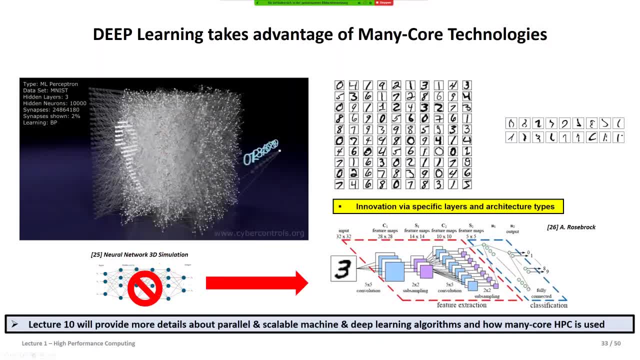 connection, for instance, but these are all details which don't matter so much. but all of these different connections between these neurons, which are modeled like the human brain neuron, really are able to learn over time. certain weights, and these weights influence then how you compute certain elements in the neuron, and this will bring you over time to really 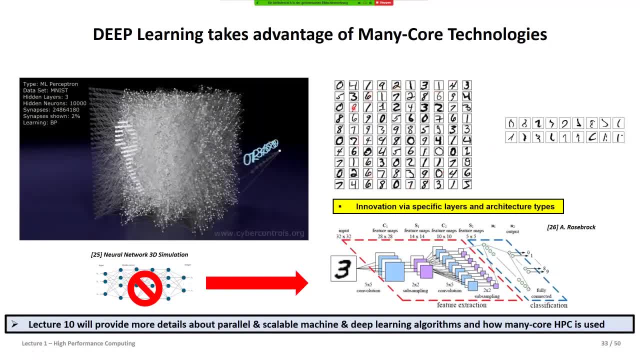 create the numbers, um, basically you can write them and this network will recognize them, except they're those you see on the right hand, which is a common paradigm in machine learning. you maybe cannot learn everything right, so accuracy of 100 in neural networks is still almost a challenge. 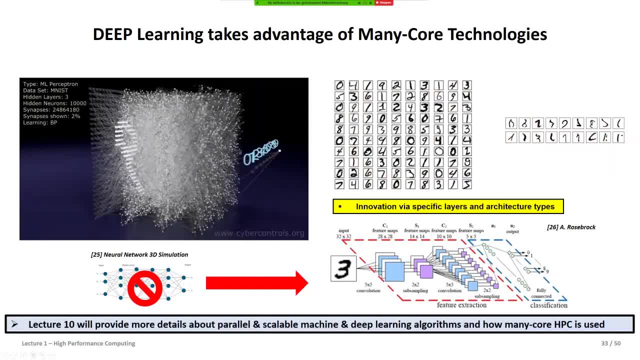 it depends, of course, on the quality of the data. nobody can really understand what was the initial rise in the neural network and then how you compute certain elements in the neuron, and then how you compute certain elements in the neuron, and then on the right hand side, I think maybe. 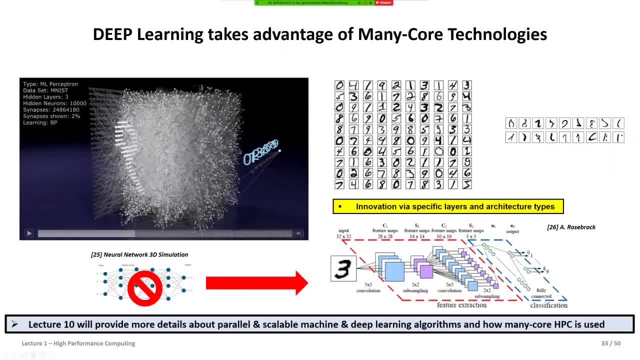 these are some of the aspects of this number right. however, one step more I want to bring for you is that this computing was already massive, but not necessarily something which you know was now limited in the past. now when we have deep learning, this new word, this is really driven now by the 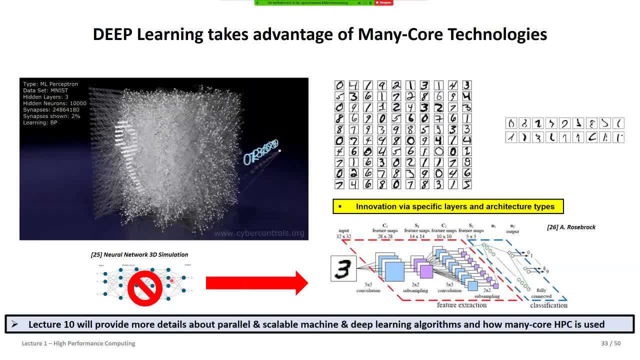 many core technologies, you would have a different type of layers. you see that a little bit here. instead of doing just neurons, interconnecting them like you see here- you will see soon in the video- we into different feature maps and these are all convoluted with different subsampling strategies. 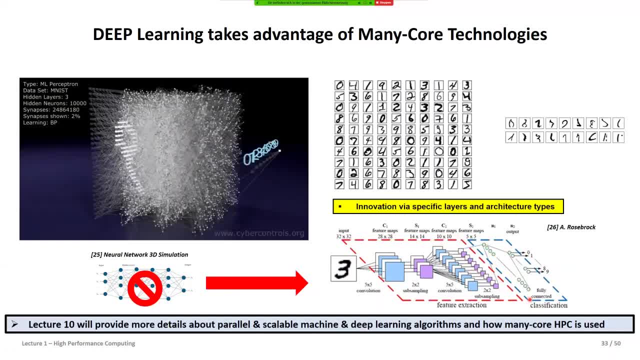 until you come then to a decision in the classification layer, And this means there are lots of computing in the, let's say, middle of this convolutional process, from this convolutional network, so to speak, which actually are on the orders of magnitudes of, let's say, 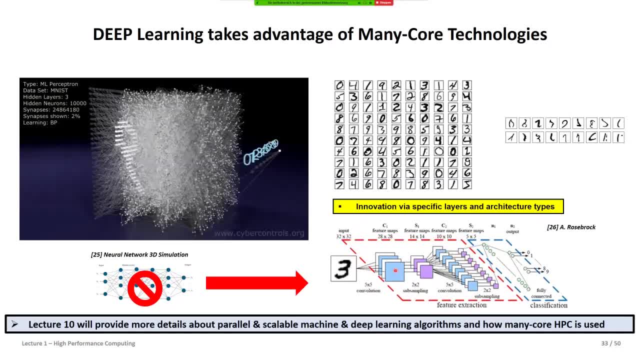 connections to be computed, especially if you think about that, you have several of those layers. Here's a very, let's say, shallow deep learning network, if you will. Usually you had the things like ResNet-50, we will see in one of the lecture had a lot of connections with parameters like 26. 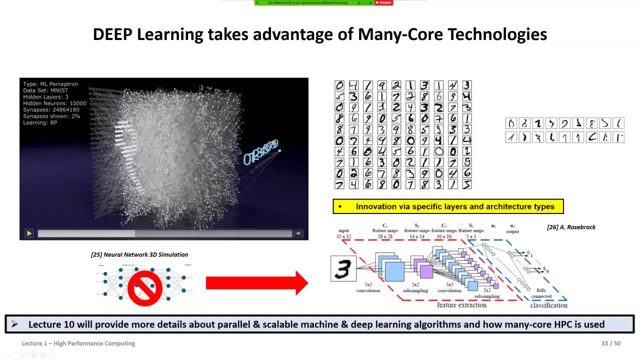 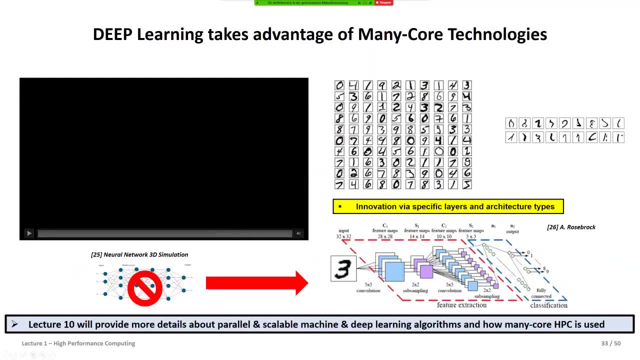 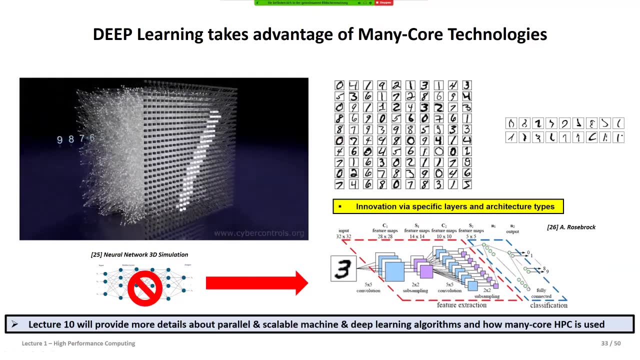 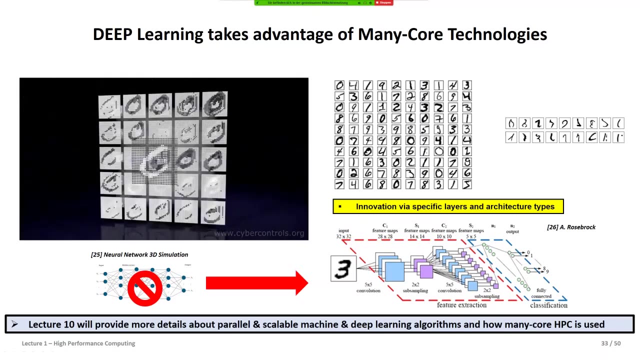 million to learn really. So let's see how that looks a little bit in the video, but more the details are then really given in lecture 10.. Again, this was a neural network we talked about with the different layers And now we're moving to a deep learning network. We see the strategy fundamentally changes, We not? 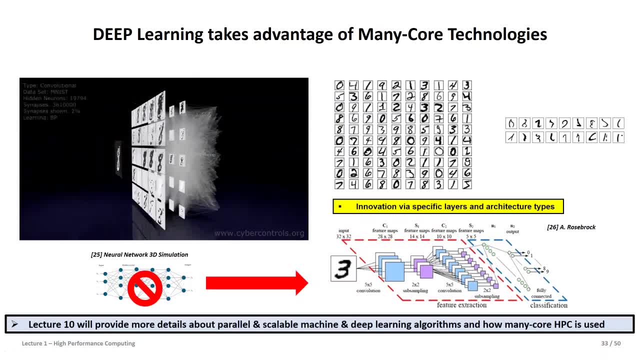 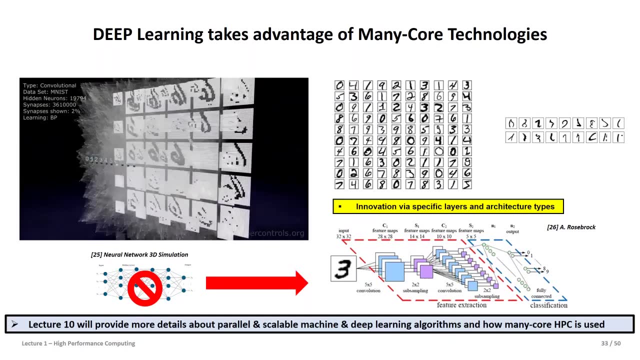 only have just connections. we have so-called feature maps, and these will also then, with different, let's say, windows, look on the properties and will identify certain aspects of the image, and we'll broke it down to more and more smaller pieces, And it is quite fascinating. 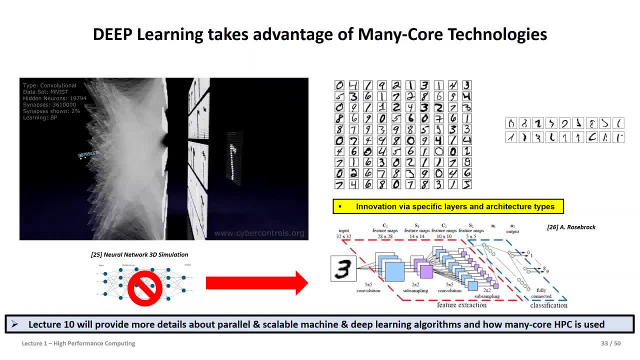 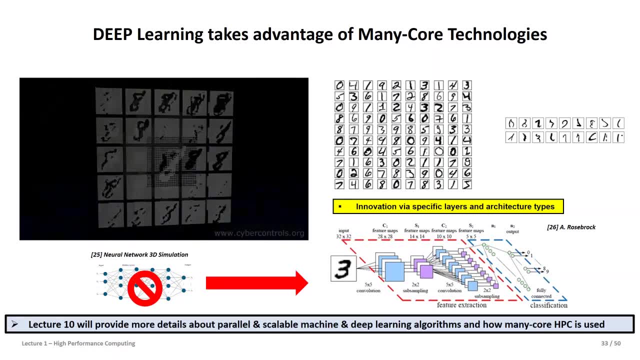 technology. but you can see that today this deep learning network is very, very, very powerful And the type of learning is only possible because we have many core chips And the new technologies which will come will have going to be one level further, But we talk about so-called spike neural. 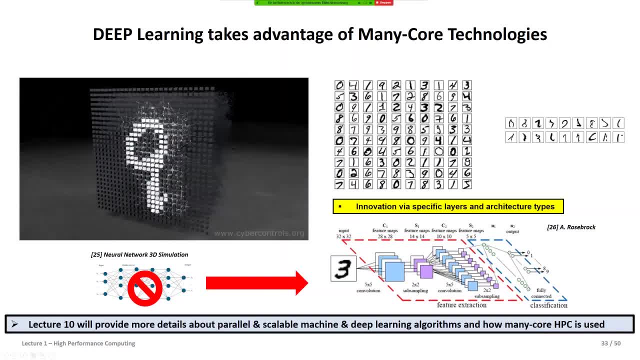 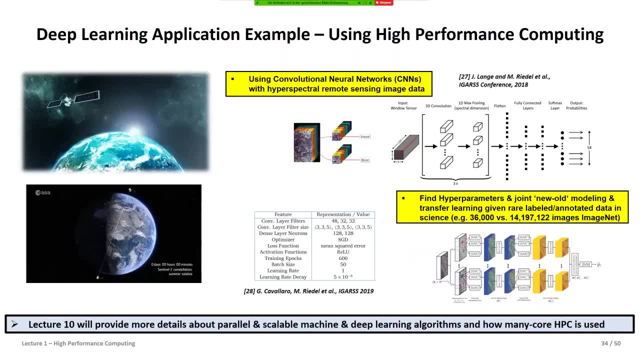 networks, which we don't really have to talk right now. It is a really, let's say, advanced way of computing this and will be also more explored in the future. So in a way, that's really what I want to leave on the table for you, for the deep learning. 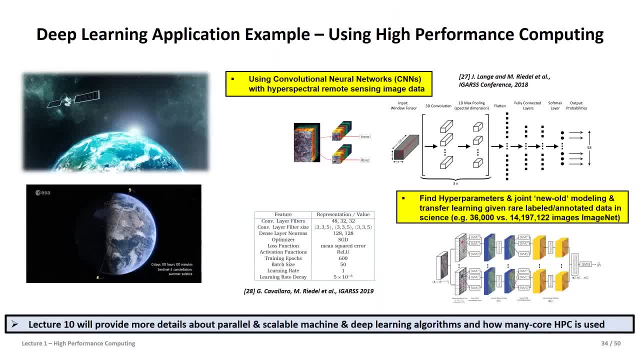 Now ways how you create those deep learning architectures, and it's another example that gives the complexity i want to allude to and why hpc is needed. first of all, you can imagine that satellites that you see here in the remote sensing area really continuously are up there. 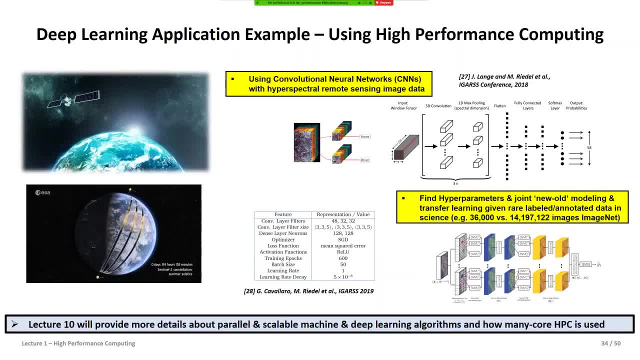 and creating generous, you know, multi hyperspectral data set, which refers to different spectral channels in the earth, data sets, and this on a 24: 7 basis. so essentially, we have big data at large which requires computing to be understood, to have, you know, deep learning to analyze it. 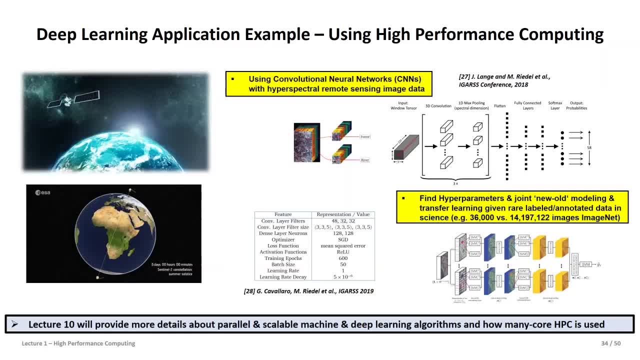 but that also means that you need it for different data sets, for big data, and this means hpc. however, what it's not really perhaps for everybody understandable yet is also the hell amount of parameters that go with it. you see here features from a certain specific- uh, basically, deep learning network. you have lots of optimizations. you have lots. 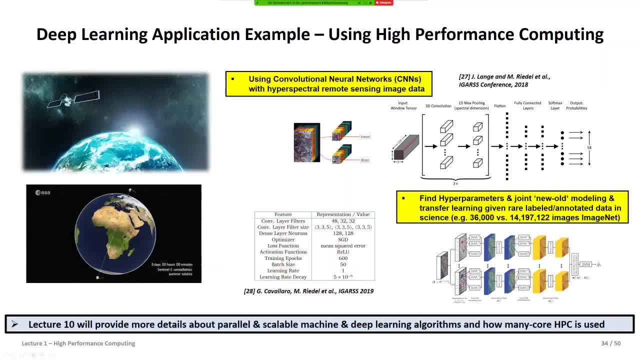 of, let's say, meta parameters to this, neural networks which require, you know, an identification. you don't know it by sure hand directly, so you play around with these parameters. you play around with meta parameters, you change the optimizers in these networks, you change certain activation functions, maybe. 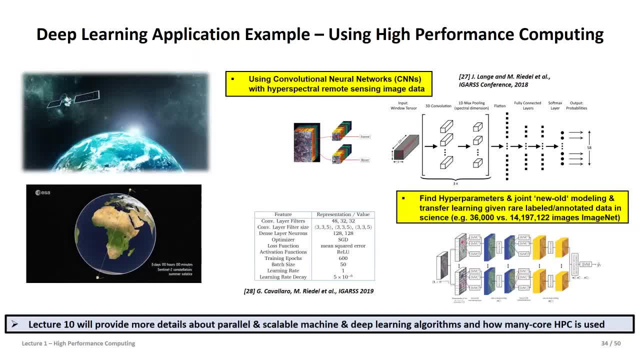 you change also then the number of layers or the convolutional layer filters and the features that you need to map and the feature map sizes. so all of this requires you to recompute and recompute and recompute right. so finding hyper parameters, meter parameters, is basically one of the most. 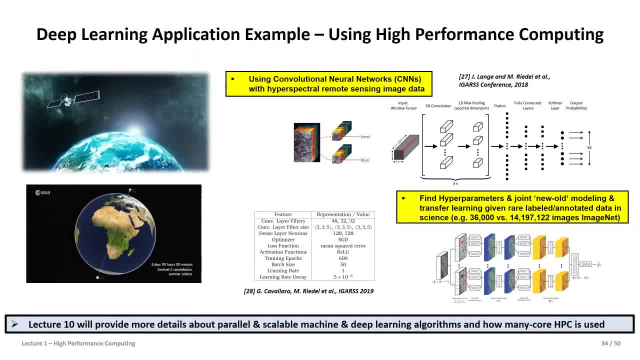 challenging aspects today? uh, in, basically machine learning and deep learning, because this really is compute intensive and there's not a really directly principled way of doing it there. evolutionary algorithms: there are, um, let's say, neural architecture, search approaches towards this in a, let's say, automated or semi-automated fashion, but still it's not, let's. 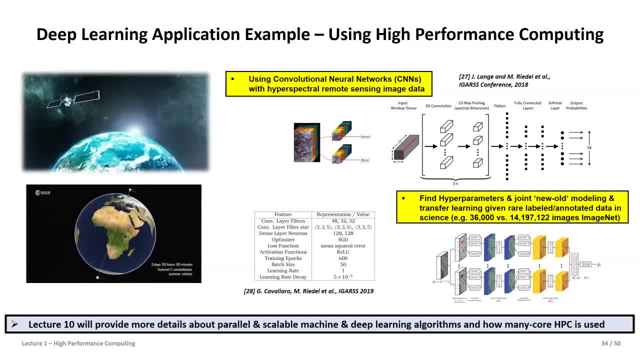 say perfect, and that's why this hyper parameter- finding those- is really a kind of another computing challenge that you see. so hence you see that, apart from all the physical simulations we maybe started in the course with understanding the stress on an aircraft, for instance, we see also that ai is now requiring lots, of lots of different, let's say, computing for different. 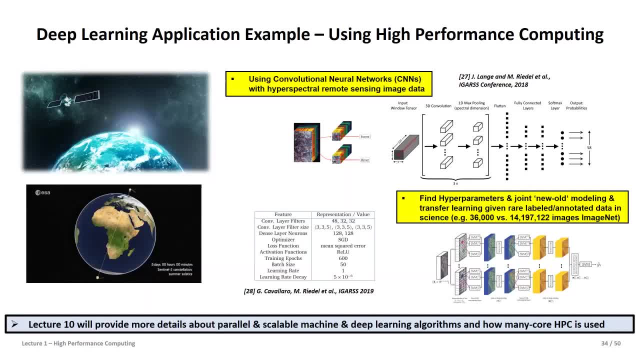 purposes, not only the data sizes and maybe also the velocity of the data. so how often i have something new when you think about the satellites rotating around the earth every time, every day. it's also that we have not completely always the idea how this deep learning architecture should. 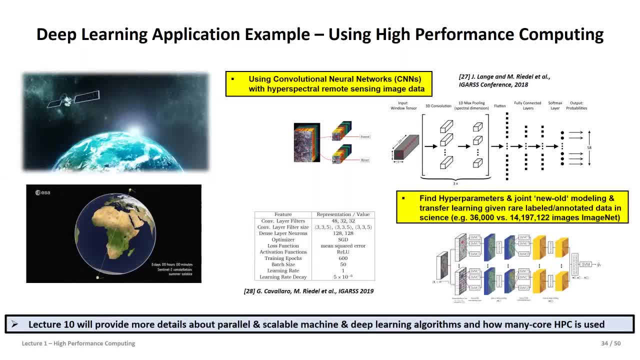 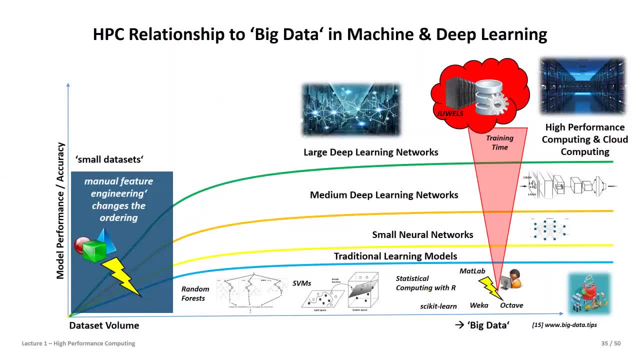 look like, and this is something which we will learn in lecture 10 much more in detail now. let us come then to the relationship of hpc. briefly, because in lecture 10 we will read this a bit more. you could say that in the past you always were this traditional classification, seems, and 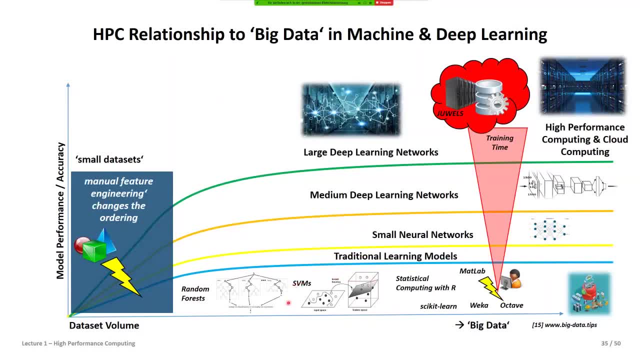 clustering machine learning algorithms quite safe. you have to use some serial computing with sky kit learn or with r or matlab, veca. these are all more serial packages, although some of them have extensions, like matlab. they have a parlor extension, but basically i've used traditional learning. 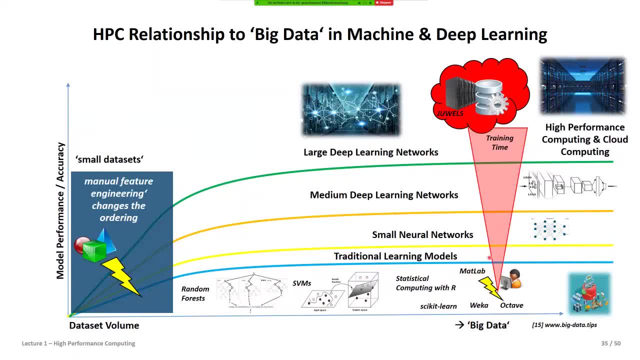 models and the impact in compute. this is the red footprint right for training those models, for working on these models. it was quite low, but now, as you come to the arena of big data and then using it with cutting-edge deep learning networks, then you see that the 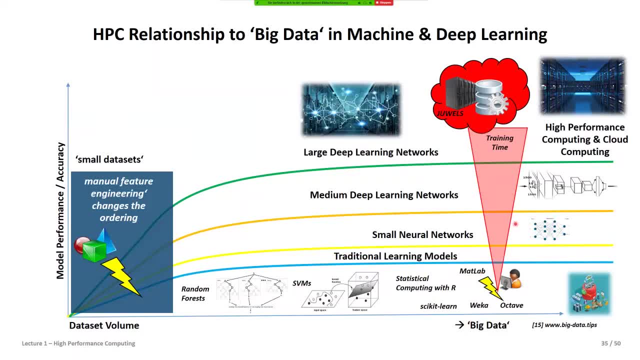 footprint in computing gets extraordinary high. so here you are in the sphere where really systems like jewels are really required and large gpus are really basically large numbers of gpus are really required to work together to really train those systems and then use it with very high accuracy in your applications. so this is really something we will look back and come back. 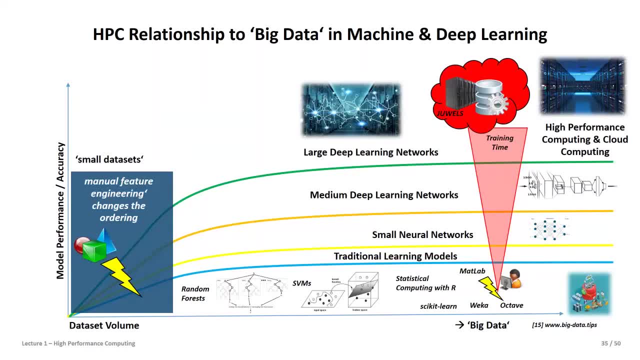 and some of you know already this a little bit from the big data and cloud computing course, where we talk much more about machine learning and deep learning, like in this course here. that's why, of course, this part has a big impact already also in the big data course and the cloud computing course. 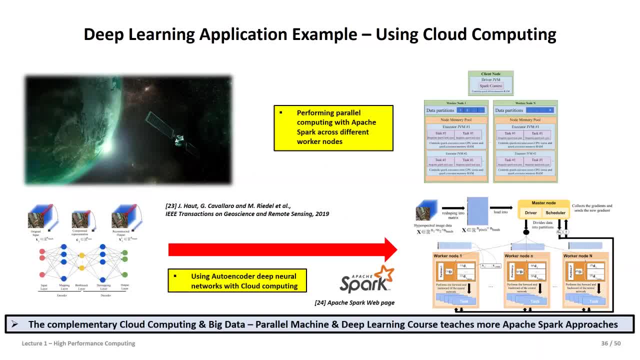 so and also this is why, basically, you could think of there's another world of power computing, which we have in the clouds, right, and it's a topic which is, of course, these days more and more getting intertwined with high performance computing, but still has a different paradigm. 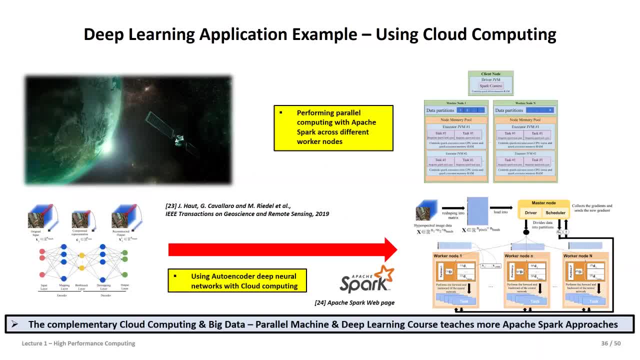 and you see here one example where we use such cloud systems with an apache spark system, which is basically a specific system for big data analytics. often, or basically in most of the clouds, in ms azure and amazon web services or in the google call up and google cloud environments. 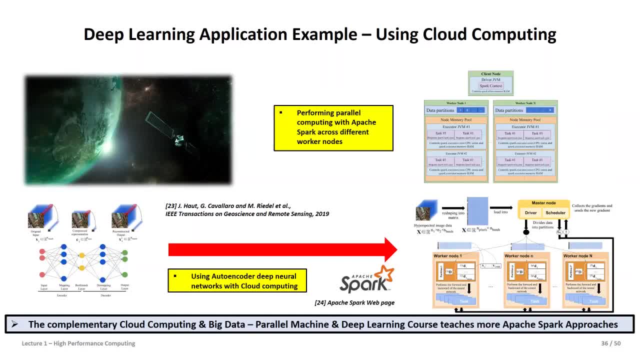 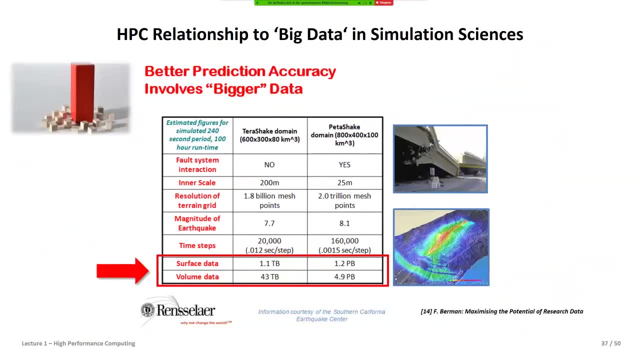 and google cloud platform available, but this is things which we actually have much more revealed in the other complementary course of big data and parallel machine and deep learning. so why is basically this now, with big data also a part in simulation science, as you can imagine. so when we want to have an earthquake simulated, for instance, that should be accurate in the past. 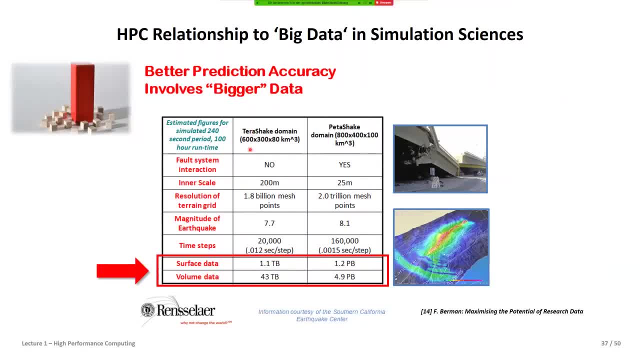 we were doing this. this is so called terra shake performance or terra flop performance, and in the peta flop performance, we can also use this to simulate earthquakes and we can also use this to- And we come to this flop notion actually in one of the next lectures- floating point operations per second. so how fast we really are. 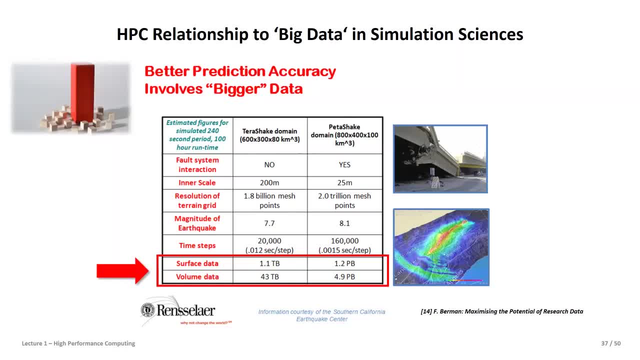 And we had this in the beginning of the course again, if you remember, with the laptop starting, then over, going to the different blue genes and then over to the cutting edge, which is now exaflop performance quite much. But the key effect that you see here by having more and more computing means we compute more and more data right? 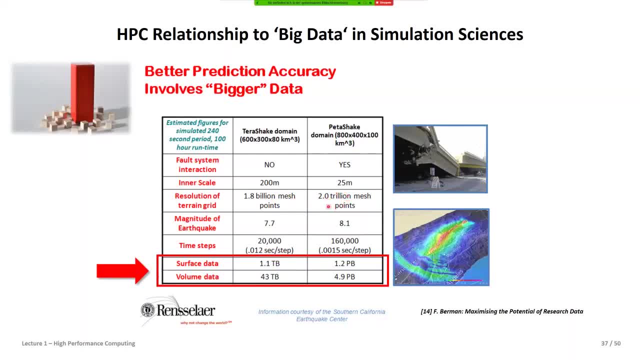 We have these different meshes. If you think about the idea of how accurate you are, how accurate you would basically have here basically a simulation from San Diego, really, basically from the San Diego Supercomputing Center, really an assimilation which actually performs, of course, on a much more detailed fashion. 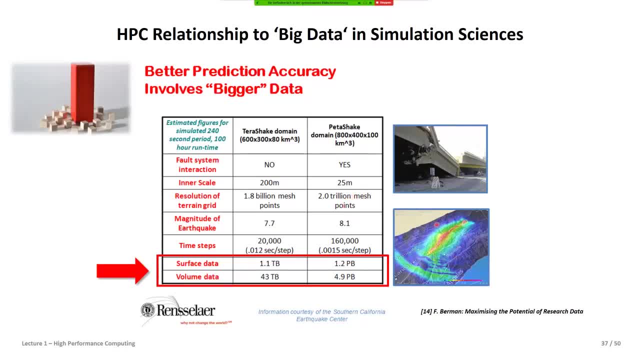 If you increase the mesh sizes of the points where you simulate, but this is where you also pay the price, where you have, then, much more surface data, rising from terabytes to Petabytes, And this, of course, also true for the volume data, If you think about we also considering things in the earth when it's about earthquake. 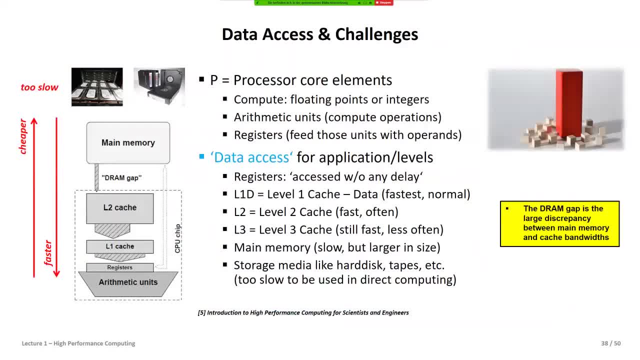 And this means also that in these days we think about data, big data, much more, also on the HPC areas for simulation sciences, And the trouble and the challenge we have still today to make this really- let's say it's extreme fast is still the idea of this drum gap. 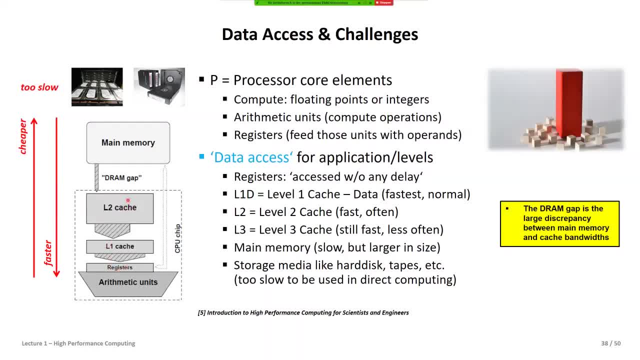 So we would have the problem that the caches and the registers are extremely Fast, but also a bit, let's say, not so, not so much in terms of storage. So you have to go to main memory and there you lose already some of the performance. 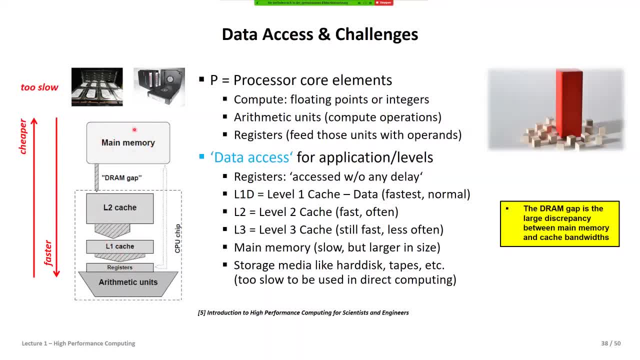 However, it's more affordable And even then you know that memory costs a lot. You have to back down to disks or even tapes if it's long term archiving. So all of this to get this into the CPUs, into the arithmetic units, is a long way, if you want, and a costly way right before it. 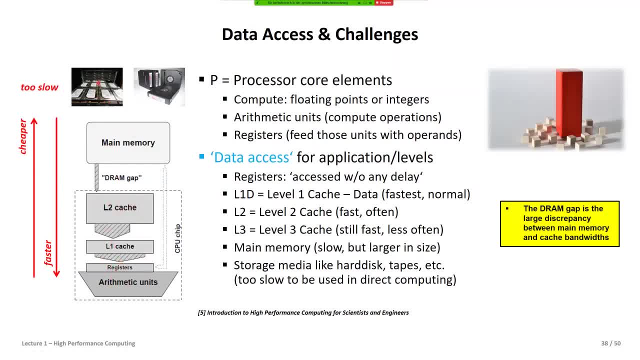 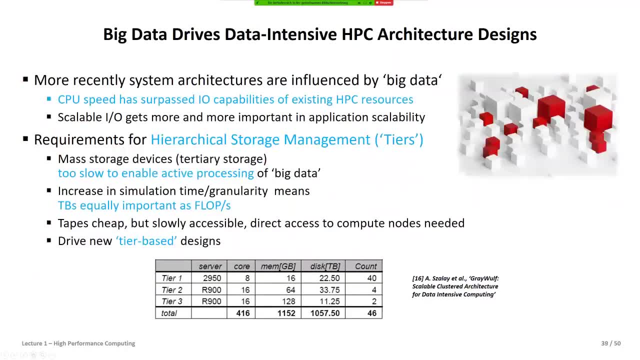 That's why the caches are usually relatively small compared to memory or disk sizes, And this is a key problem we have right now still in the community. However, we see that this big data really drives different architectures, and you see here already a kind of different modules, different tiers to do different things. 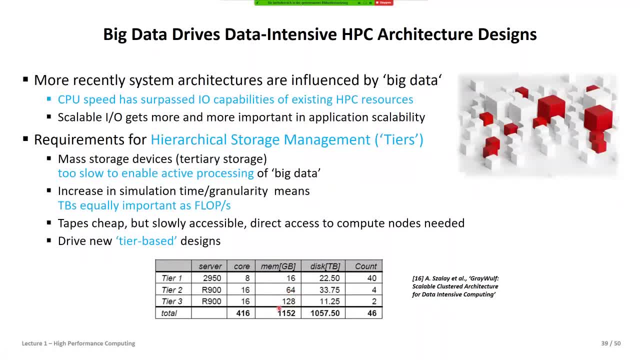 We see that more and more memory is important for certain applications, while some of them maybe just require more disk space, but then should be very many of those. So you see That basically, this kind of homogeneous system that you have is more and more looking towards hierarchical ideas, to its modular ideas We also had in the video about jewels. 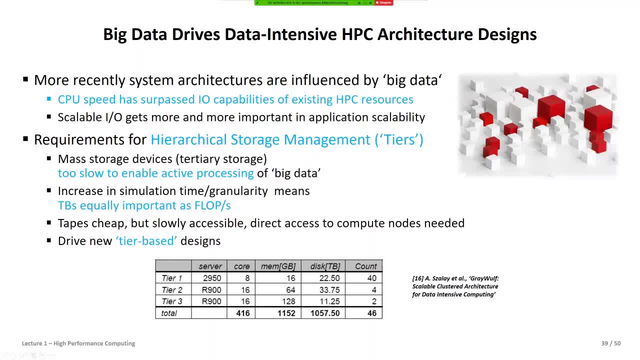 Right. So this is related to it And it's due to the fact that we have to think about the terabytes, or data in general. data intensive sciences, data intensive access to these systems is more important than just the pure computing power of flops per second these days. 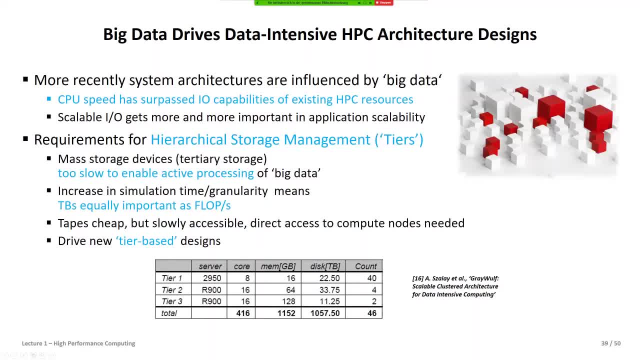 And this is drives, new tier based designs. Here's one of it. But of course there's a lot of data. But of course there's a lot of data, But of course there's a lot of data. 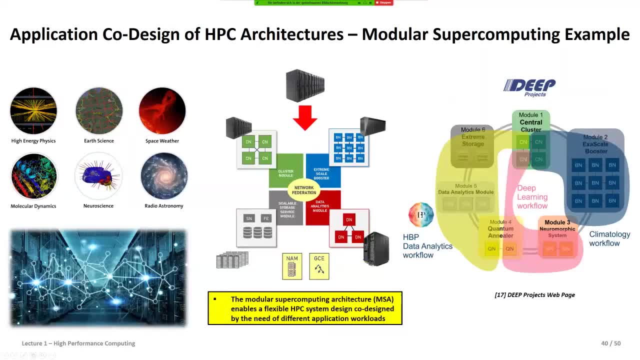 But of course also the modular supercomputing design is in a way an idea of it. You have seen in the video this cluster module with high single-thread performance booster to scale out, and then maybe data analytics module for things like Apache Spark we have seen. 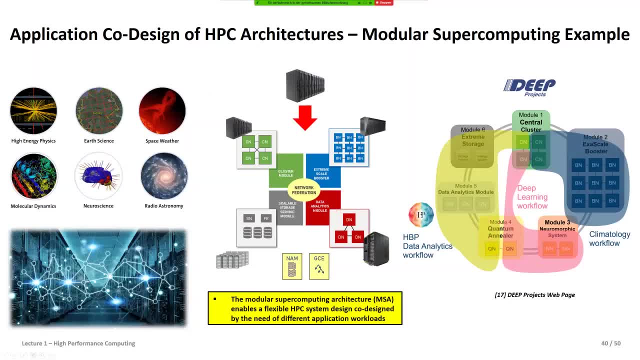 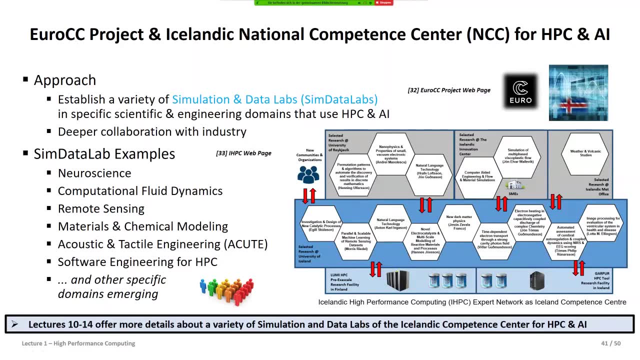 Or the more recent aspects I come to in a moment, with a quantum annealer right. So very interesting if you think about this. And Iceland was part of this, which spawned another activity which we have in the URCC project, where I want to 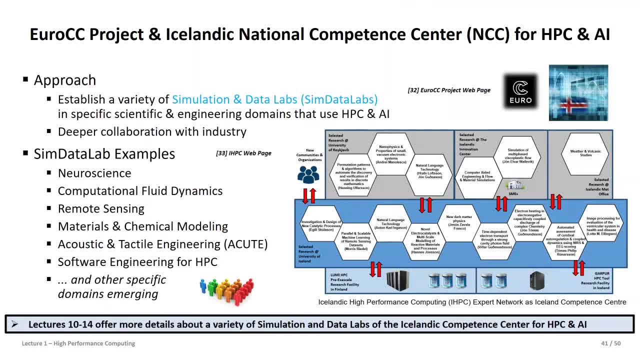 I want to also give you another perspective now of what things are happening in the future here in Iceland, what's happening in general in the ecosystem around Europe. in HPC, There's a building of national competence centers all over Europe. We are in the URCC project, also in Iceland, together with 33 other countries in Europe that create so-called competence centers. 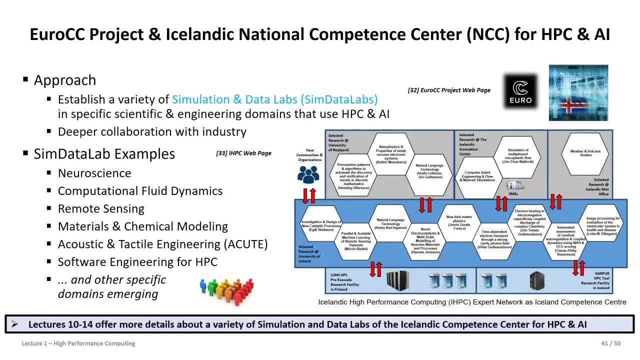 What we do here in Iceland is we establish a variety of simulation and data labs and you're welcome to perform maybe your math assays there, to get involved with some of these projects. We have some of these simulation data labs in the field of neurosciences, computational fluid dynamics, remote sensing materials. 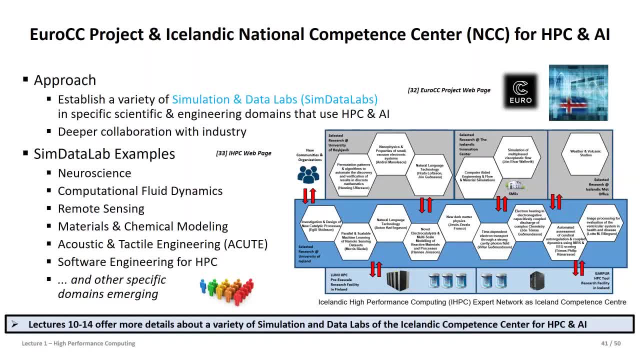 More and more we create and more and more of the scientists from Iceland, the PIs really you see here mostly working with HPC systems, are basically forming with us, those labs to be a bit more structured as a community in this national competence center together as a bottom up approach really. 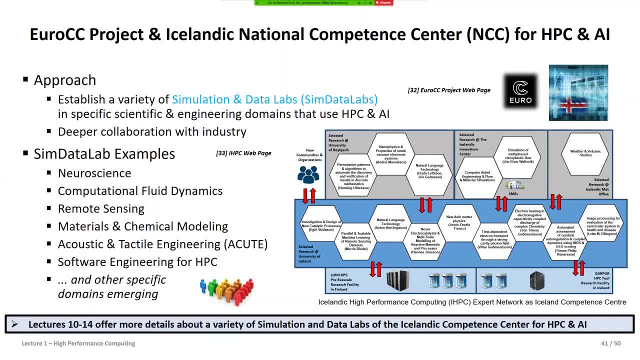 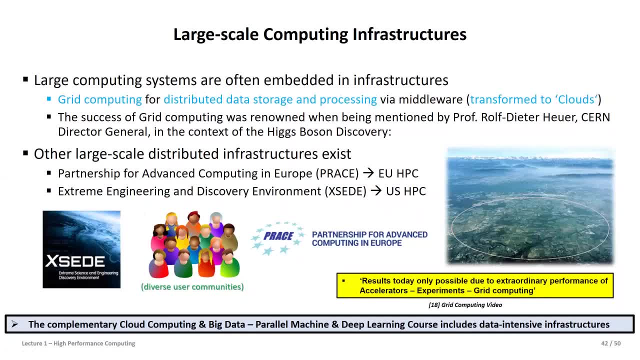 And you will learn much more about this when we come to lecture 10 and 14 and the course Now towards the end. two perspectives when you think about large scale computing infrastructures. I could talk a long time about it. I will come back to those. 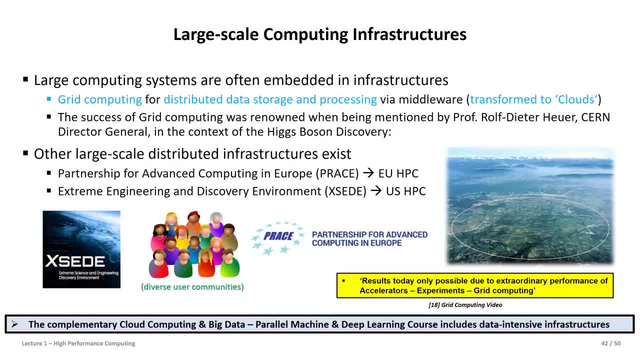 You have those of the grid computing. you may be heard in the past with the Higgs boson that was found at the CERN laboratory in Switzerland. You basically have seen that grid computing was one key ingredient and grids by far have been transformed to cloud computing, still sharing many of the parallel computing ideas we have here in the course. 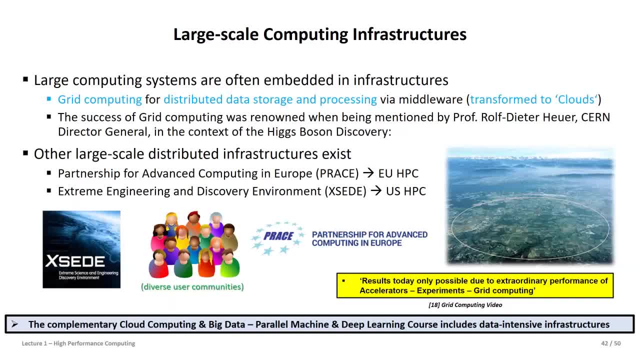 However, they're also different. If you think about distributed infrastructures, if you think by using just one HPC system, you also would consider to have a grid of those HPC systems. so not only one HPC system, but you want to have maybe the one in Italy used instead of Germany, because it has some application experts that can help you scaling up. 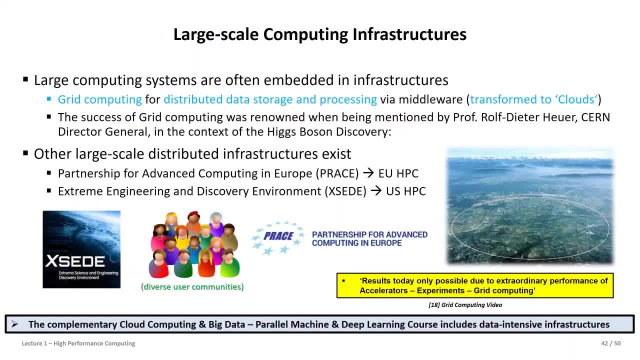 You would like to go to US because you have a particular collaboration working on some data intensive aspects where the data sharing in US might be simpler than in Europe or there's just available data in US. So all of these infrastructures- PRACE, Partnership for Advanced Computing in Europe, and also the extreme science and engineering discovery environment EXCEED in the US. what they all have in common, in a way, is that they basically have diverse user community. 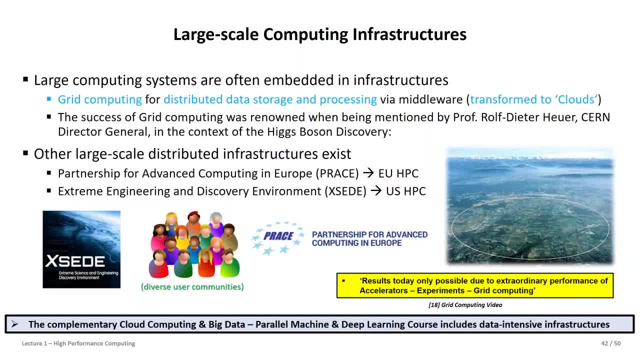 So it reaches up again from material scientists up to computational fluid dynamics, people understanding airflow, from medicine up to neurosciences and basically then also our system sciences. You will find lots of different user communities, communities that using these large infrastructures- We will come back in this also from time to time And, of course, a complimentary cloud course told much more about this infrastructures idea, like we can do here in our course in HPC. 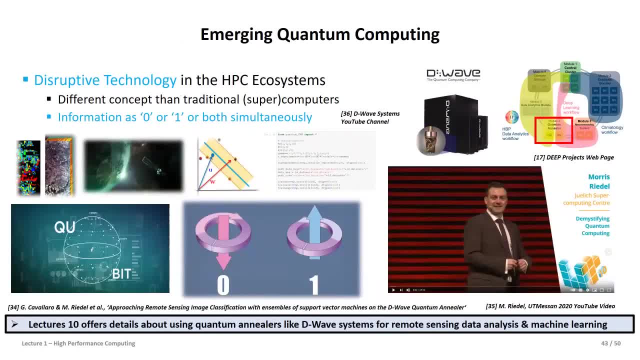 So I would like to close a little bit with the idea of quantum computing And this is loaded And of course I could have a complete lecture series about it, And we don't do this very much in the course. We will have a lecture 10, a little bit small part of it when we talk about one of our studies already, when I show you that we used already D-Wave quantum annealer. 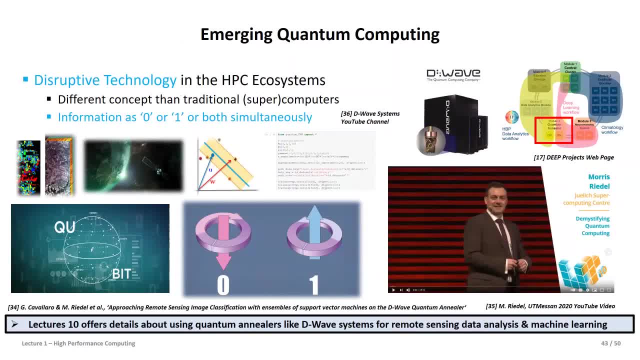 It's a specific type of quantum computing. quantum annealing for a support vector machine, a quantum support vector machine working on And then remote sensing data sets- So that works- is usually a bit different than conventional computing. Hence it's a disruptive technology. We don't have just a lot of zeros and ones anymore. 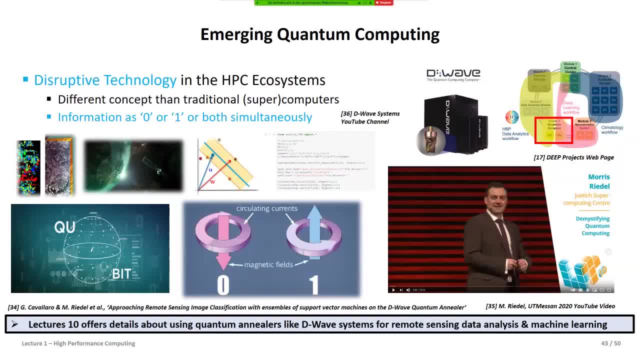 As you know from the binary system, here we're talking about actually a superposition of having one and zeros both simultaneously. Still, we compute this still and using this, if you see, here with a Jupyter notebook, still in a very, let's say, straightforward manner. 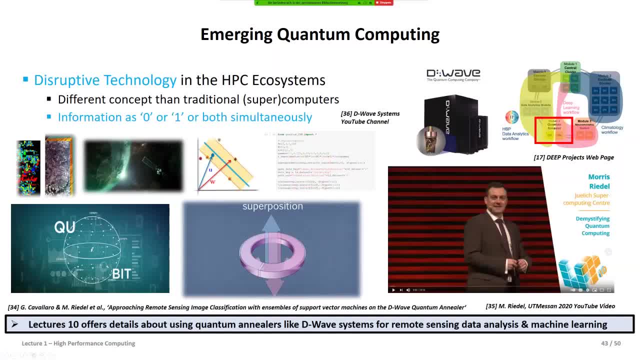 But to compute This of course requires, then, much more mathematical thinking, much more thinking about how we can break these things down using qubits instead of this typical things we know from ones and zeros. And you see, the vision is that this will be complemented with the typical things we know: the cluster module, the booster things you know from the modular supercomputing quite well now. 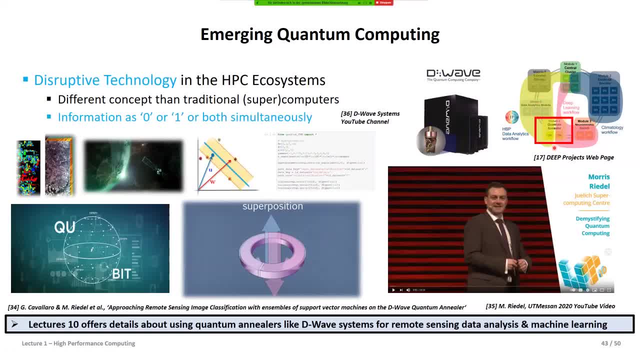 But there will be a quantum annealer in the future. Jülich is already building a building where D-Wave system will be actually Hosted, and with this you can always, let's say, use it as one part of the module. 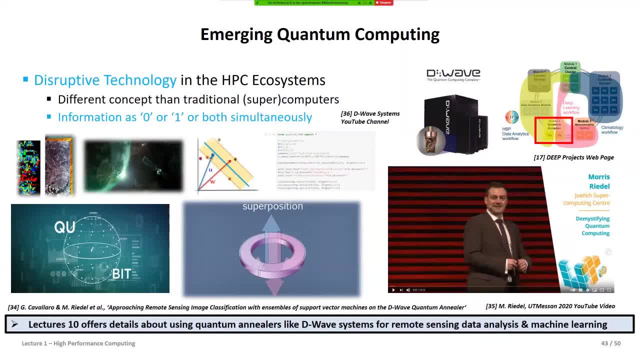 You would say some of the machine learning optimization algorithms that really can benefit from. we computed on a quantum annealer, while many other general computing aspects still require, maybe in deep learning, the central cluster, And the same is true with neuromorphic devices that come. 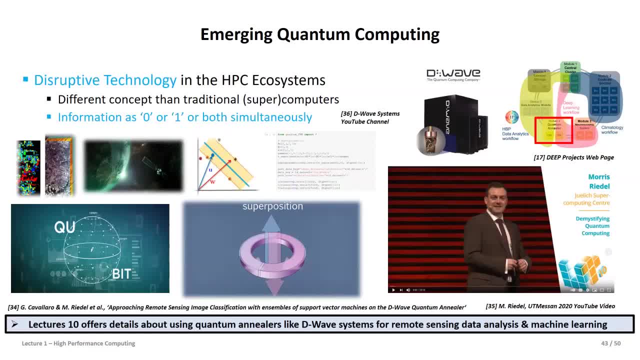 If you have interest in this area. there are of course also master seasons available. But you see, also I was invited here to the UTMessage And in one, basically last year, a kind of presentation that is available on YouTube where I give, let's say, a small introduction to quantum computing really was a quantum annealing perspective which might be interesting for you to look at. 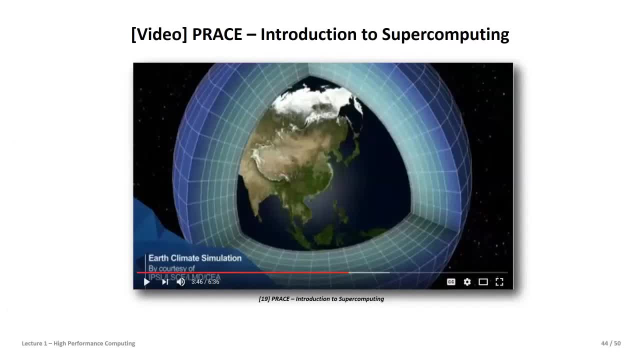 We reached essentially the end of the lecture again, so we have another video for you. If, in case, the sound is not perfectly played and recorded, you will always find, of course, a link then in this references. So let's go to the video. 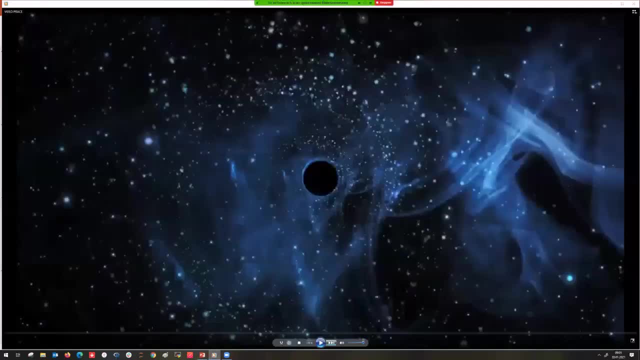 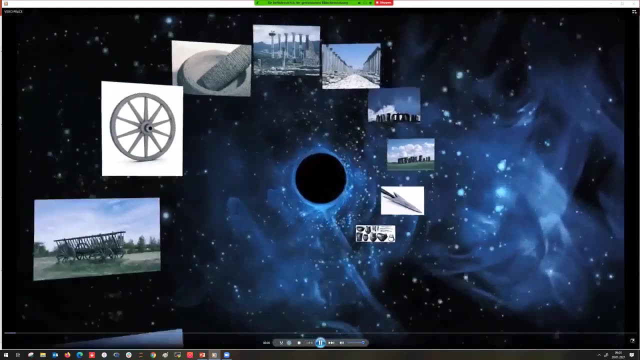 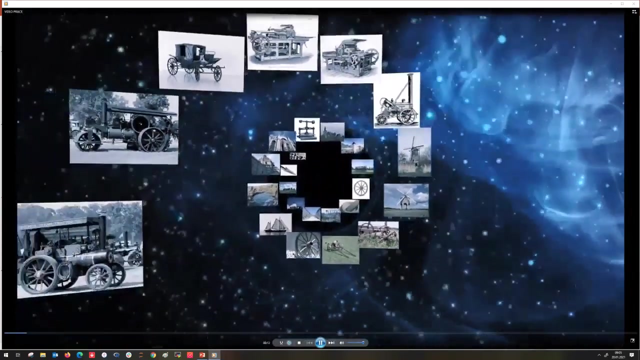 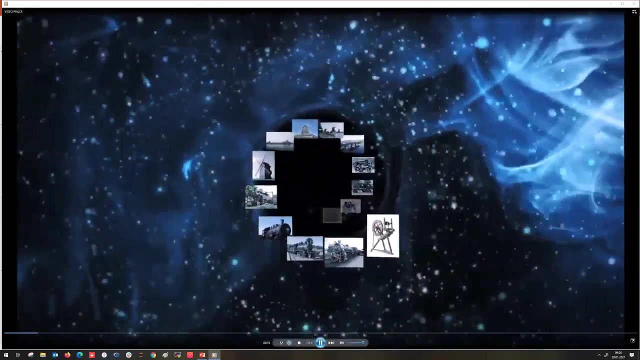 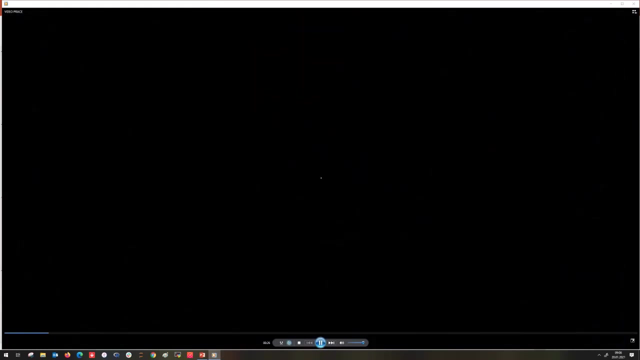 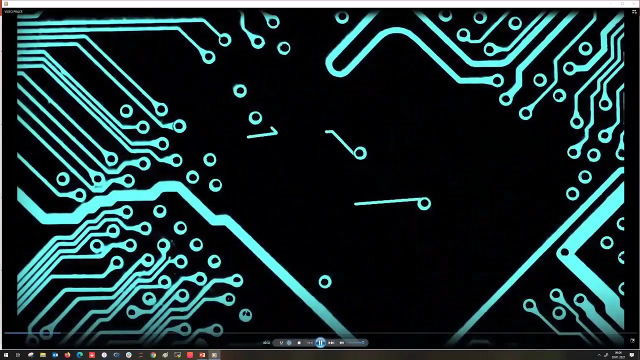 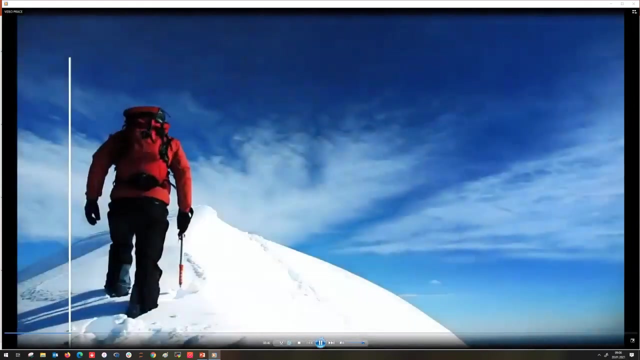 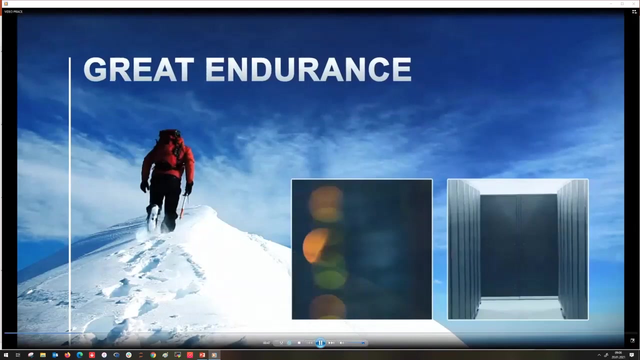 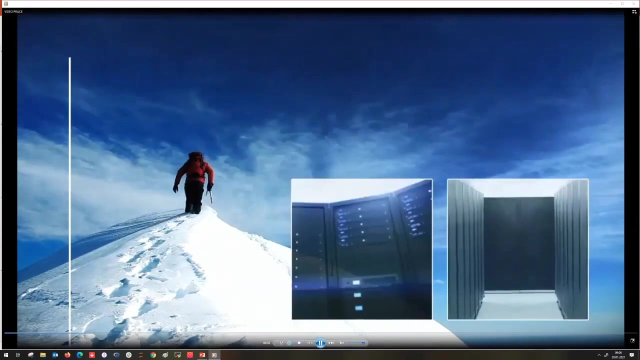 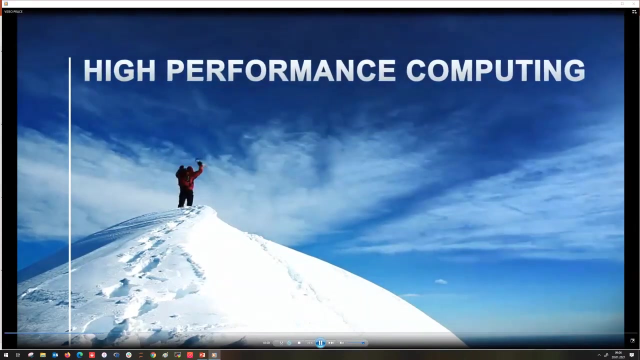 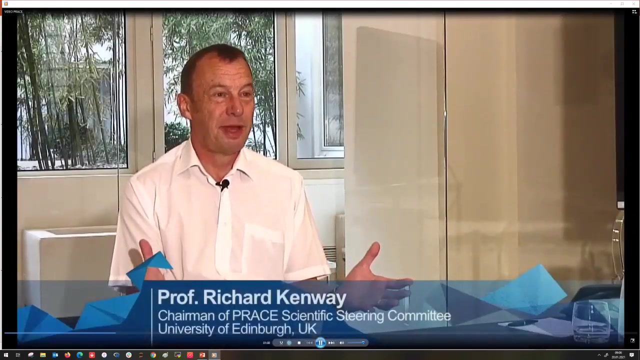 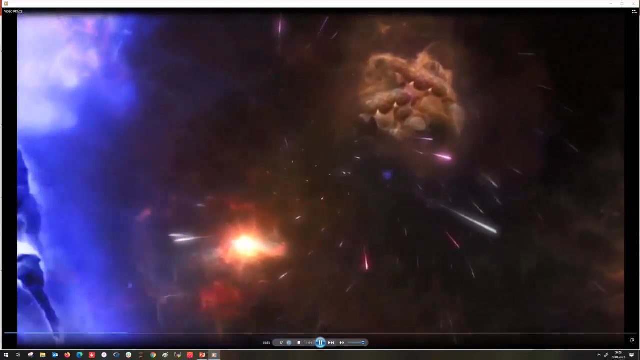 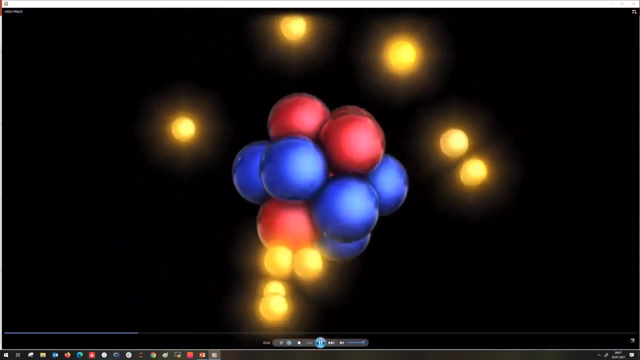 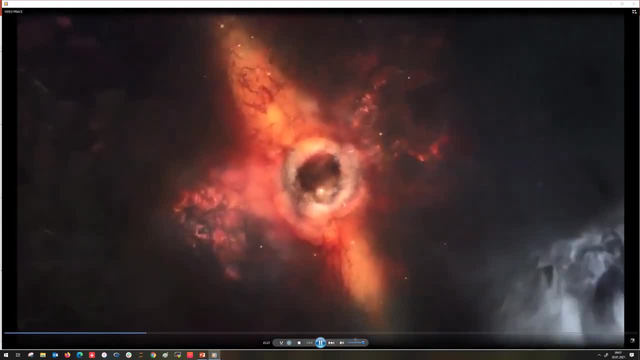 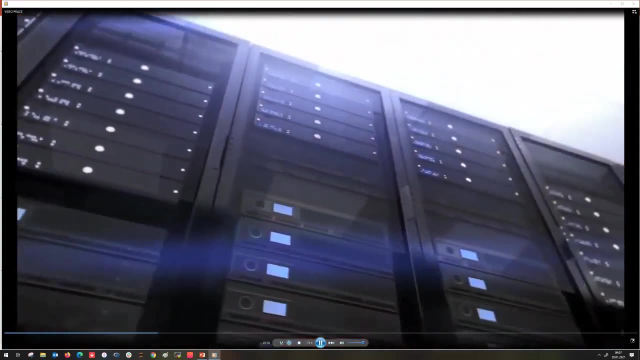 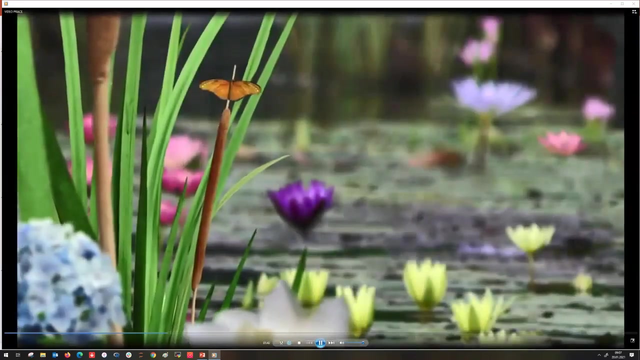 It's a reactor that enables us to study plasmas and what's going on in the interior of stars, And it's even a time machine which enables us to recreate the past or to predict what's going to happen in the future- Almost all of the major challenges that society faces. 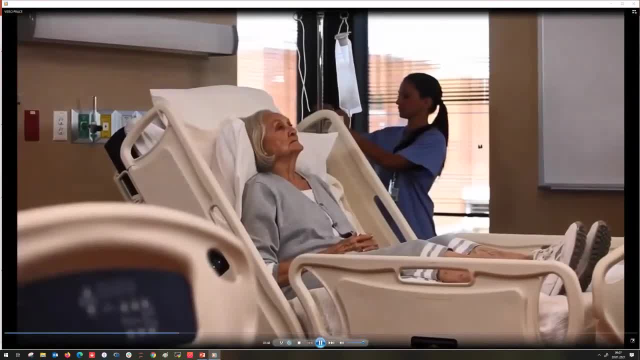 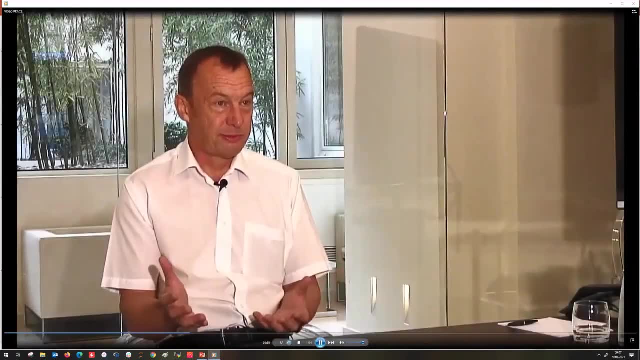 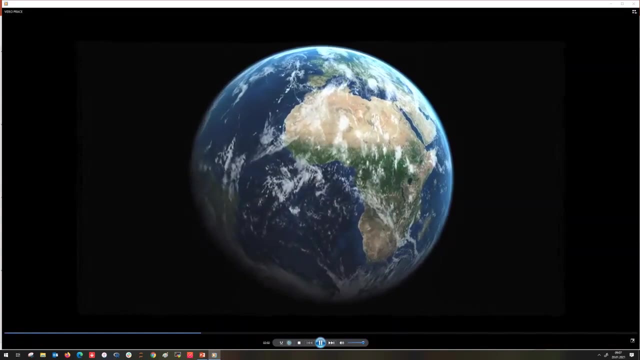 whether it's preserving our environment, improving our health care or rebuilding our economy, are underpinned in some way or another by high performance computing. By pursuing our dreams or looking for new perspectives, we test our instincts, abilities, knowledge and spirits that regularly go beyond physical boundaries. 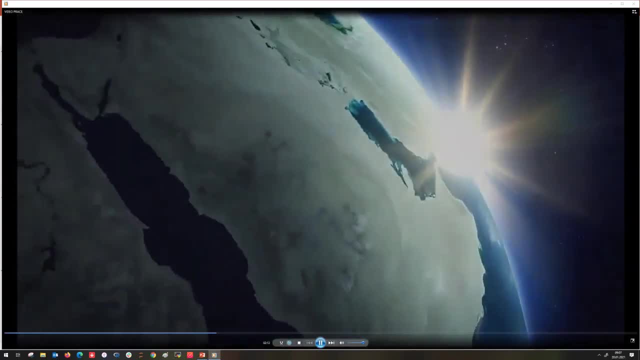 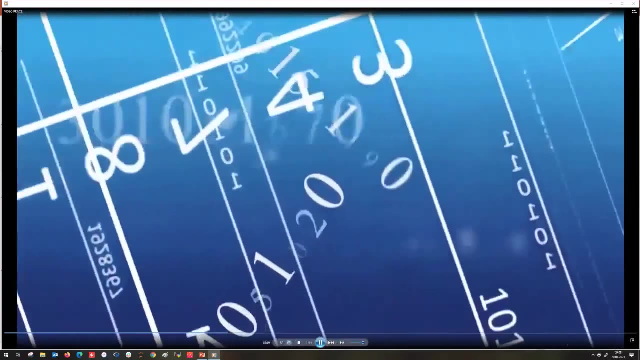 And so, if you are not a scientist, what are you really looking for? And what are you really looking for in the humanities of today? What are you looking for in this world? What are you looking for in the球 or in the sky? 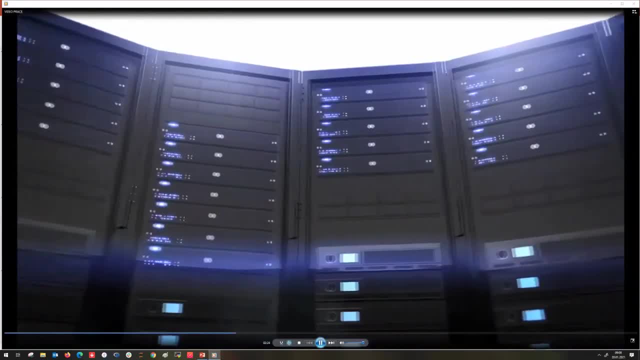 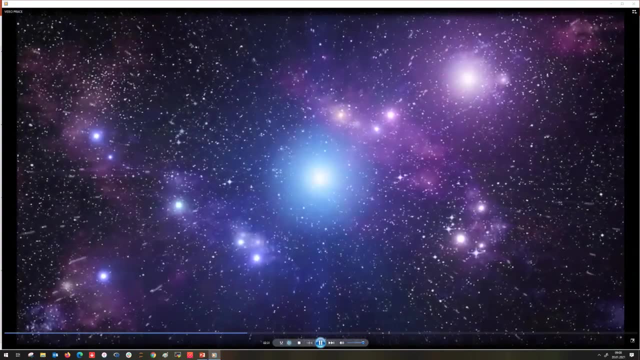 Whether it's the past or the future, Or whether you're just an internet scientist or you just have a dizziness with the science challenging you. What's your purpose in this world? What's yourlingting goal? What's your motivation? What's your motivation in this world? 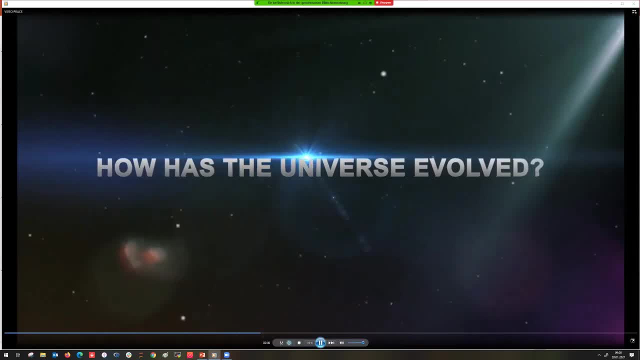 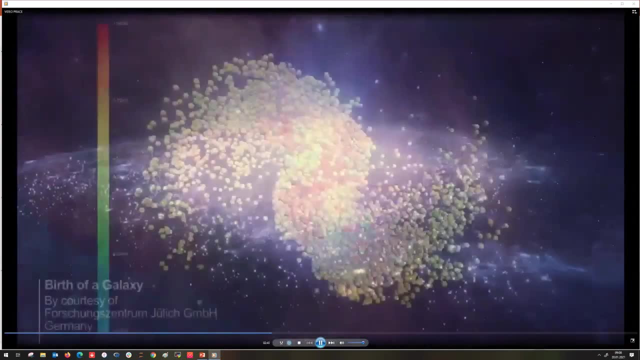 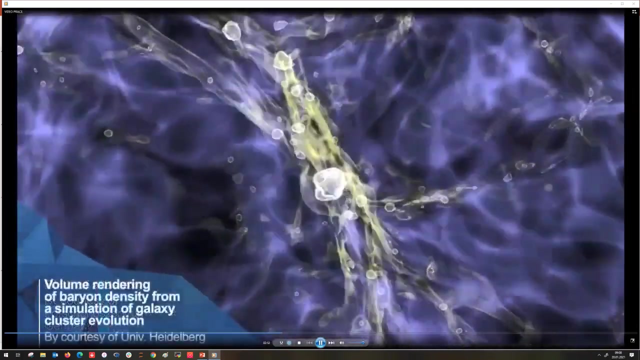 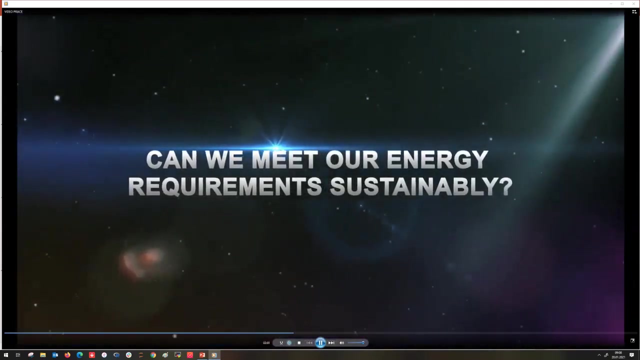 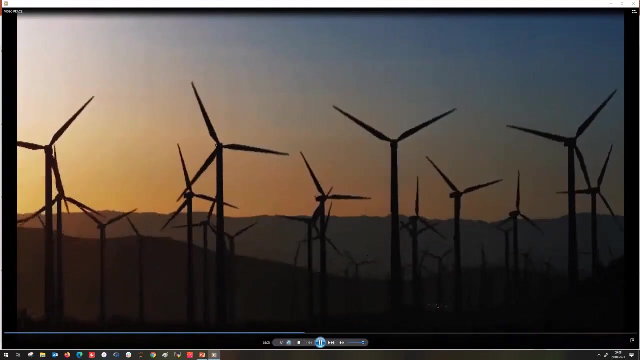 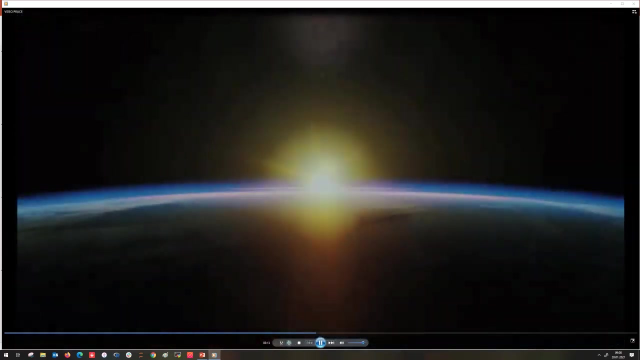 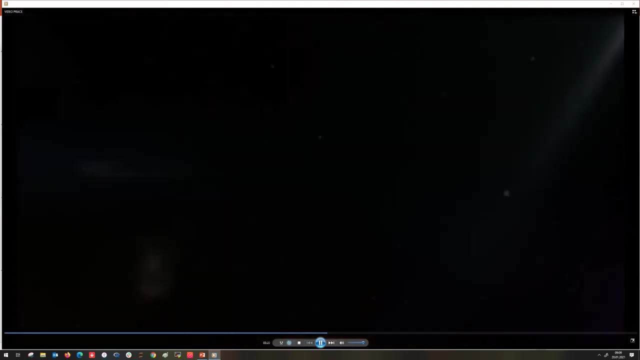 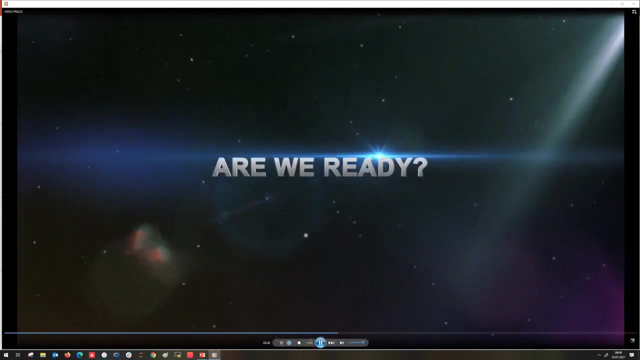 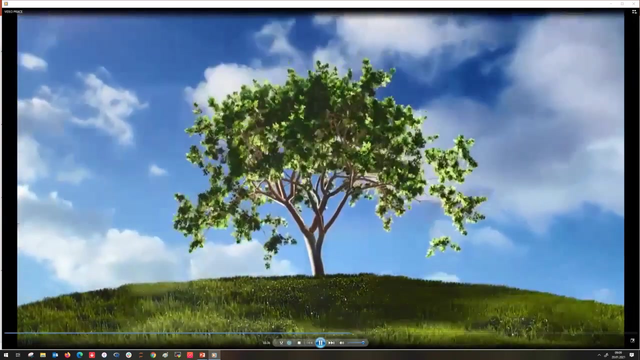 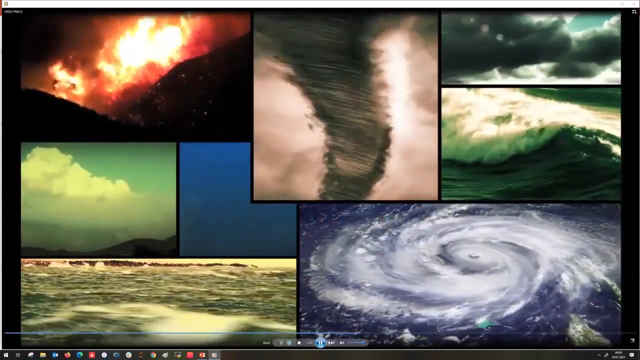 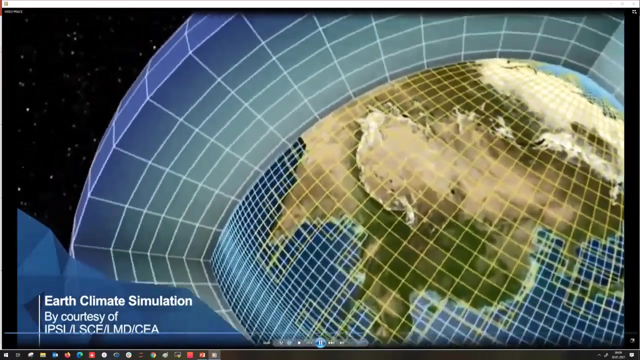 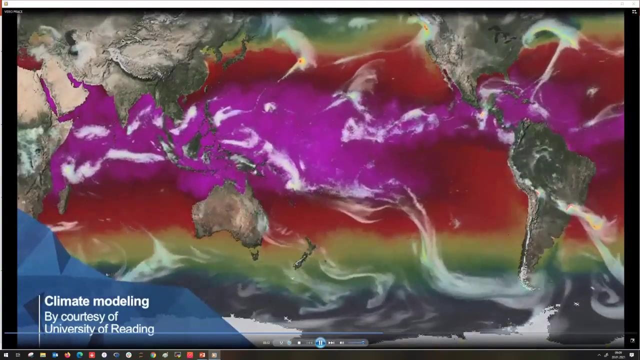 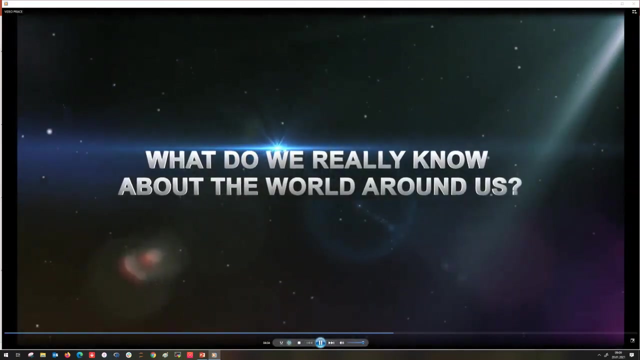 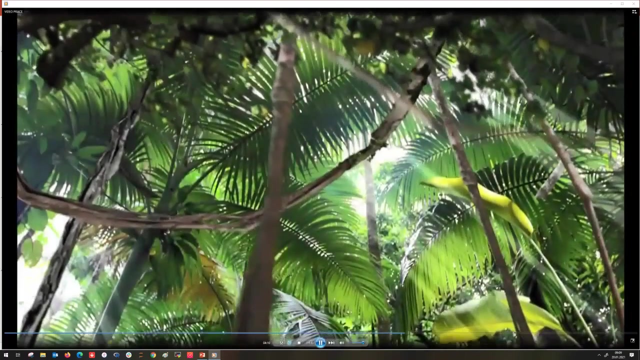 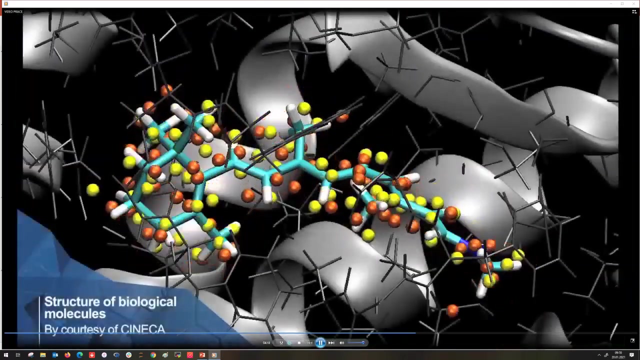 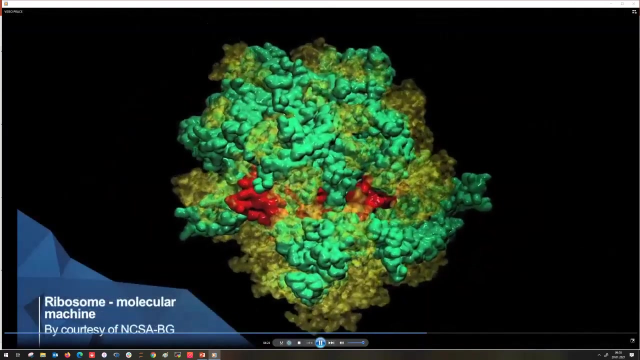 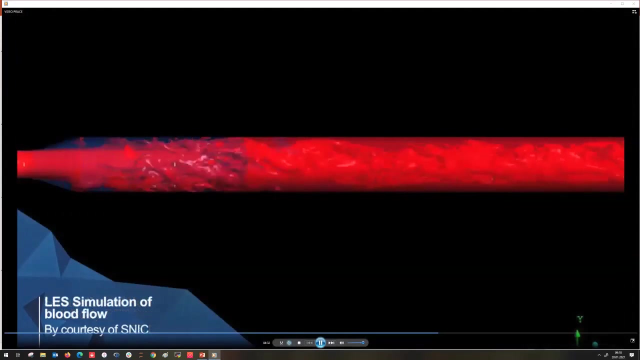 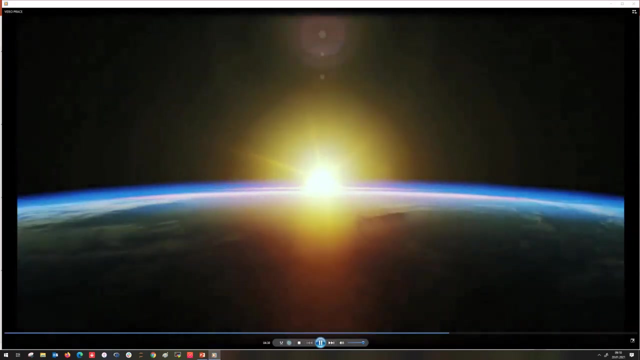 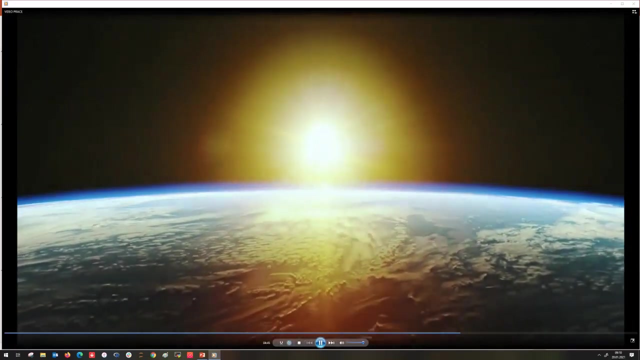 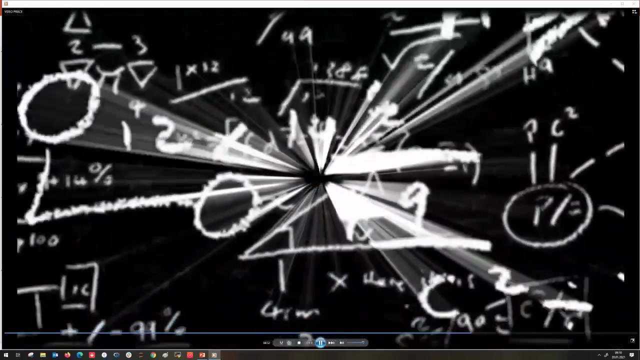 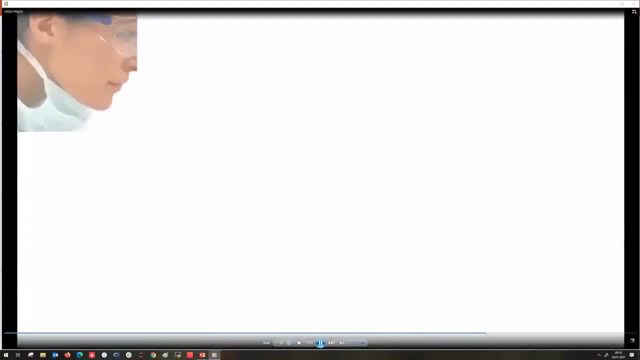 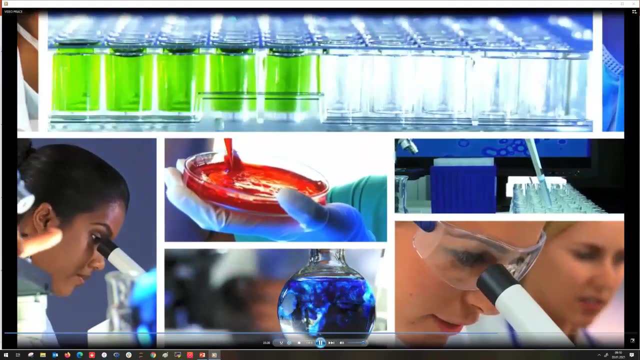 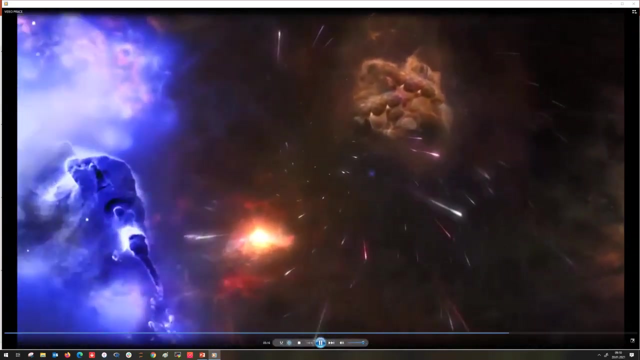 Equipped with the most powerful supercomputers. today's scientists and researchers have the potential to deal with the complexity of the phenomena by Gathering new results and findings leading to further refinement of their initial ideas, Applying a comprehensive explanation supported by many facts and data gathered over time. 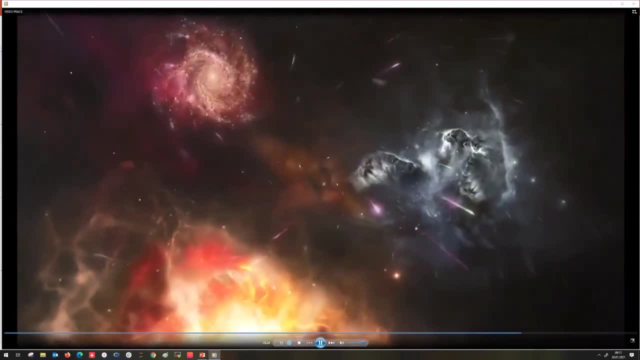 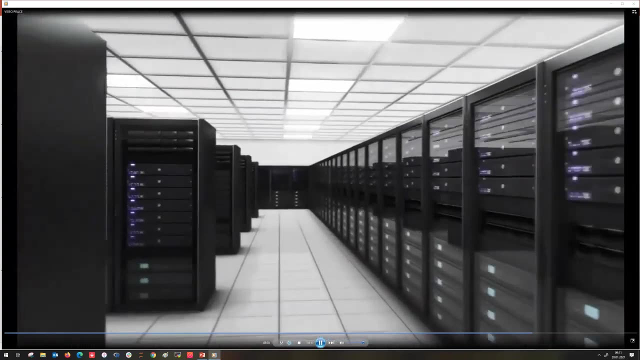 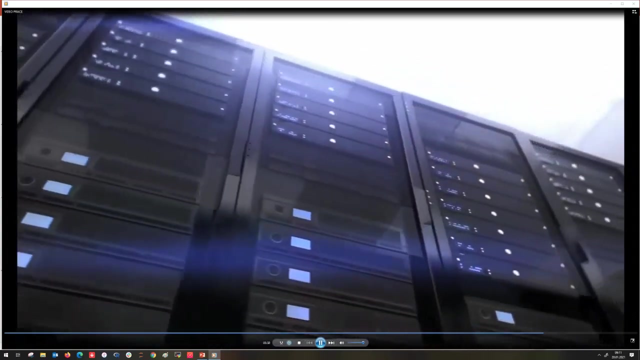 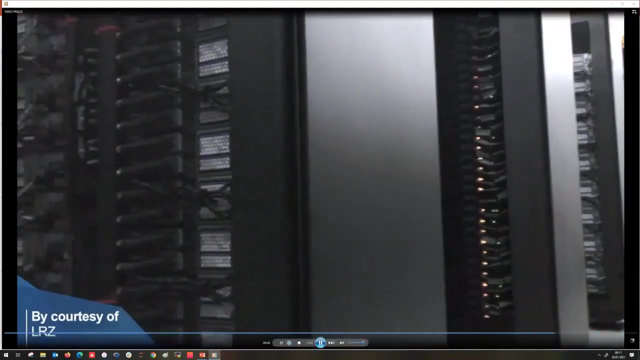 And generating new hypotheses to predict yet unobserved phenomena. Ultimately, supercomputers allow the hypotheses of our greatest minds to be explained, or even rejected when compelling contradictory evidence comes to fact. Thank you, That's because supercomputing brings an unmatched combination of computational capacity and capability. 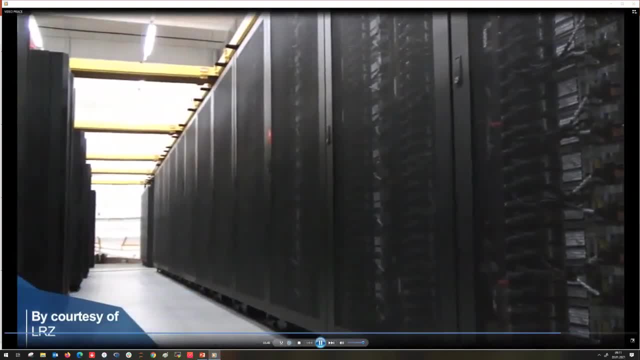 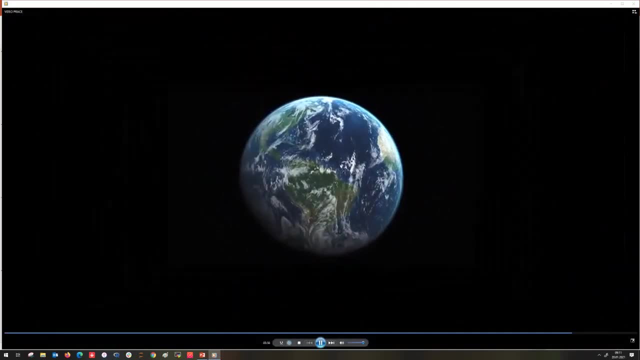 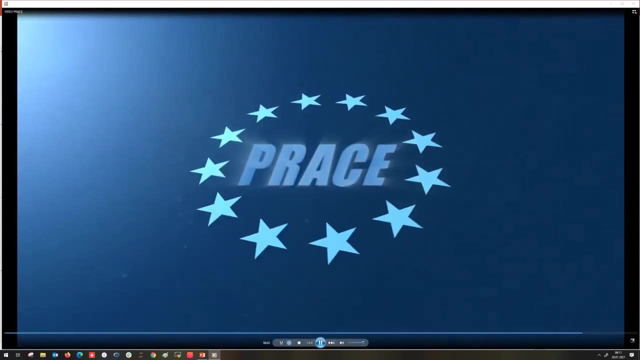 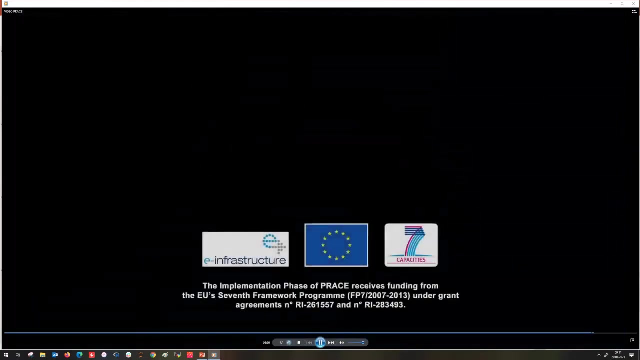 which undisputedly strengthens the solid foundation of observation, experiment and confirming evidence. We are in the process of developing a new technology that can help us to know more about the world around us. We are in the process of developing a new technology that can help us to know more about the world around us. 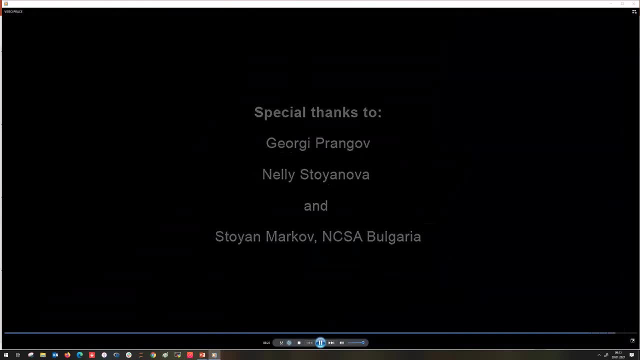 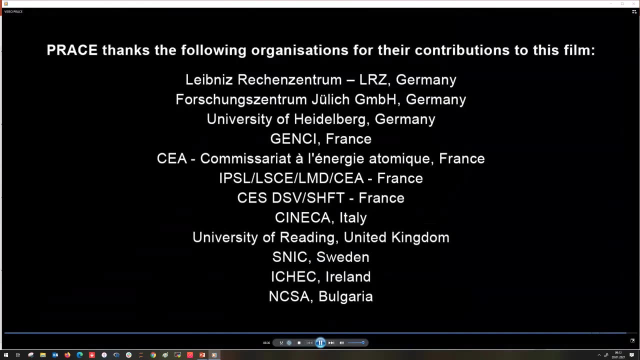